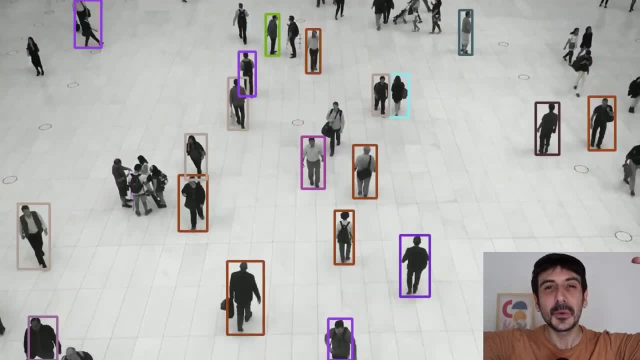 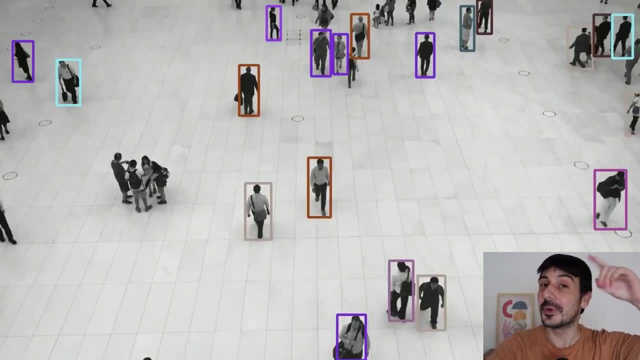 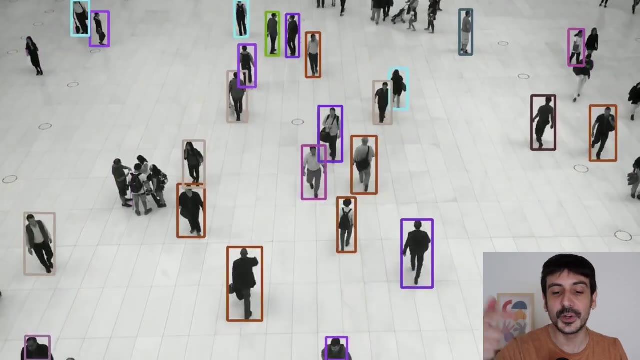 Hey, my name is Felipe and welcome to my channel. In this video, we are going to work with object detection using YOLOv8, and we're also going to do object tracking using DeepSort. So this is exactly what you will be able to do with today's tutorial. You can see that this is a video of people who are just walking from one place to another, and each one of the people in this video, each one of the persons in this video, has a bounding box of a given color. 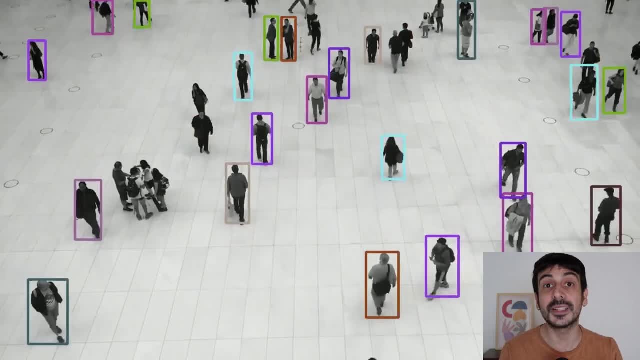 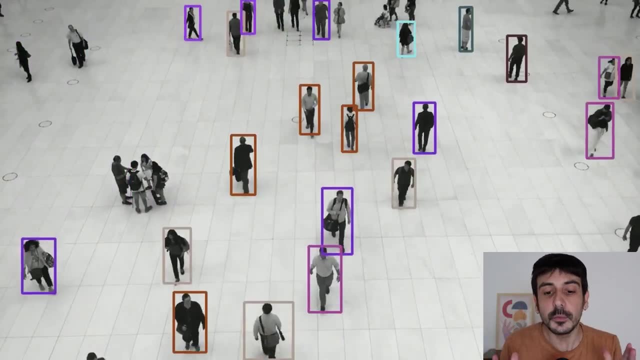 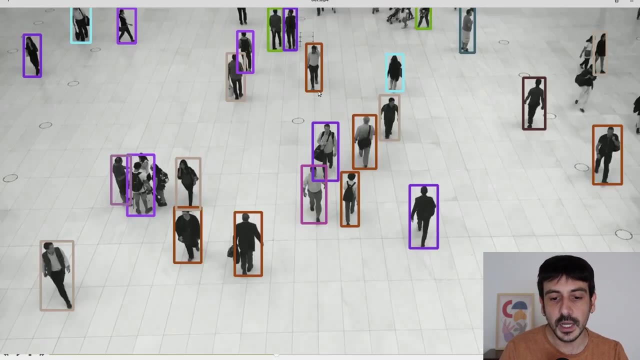 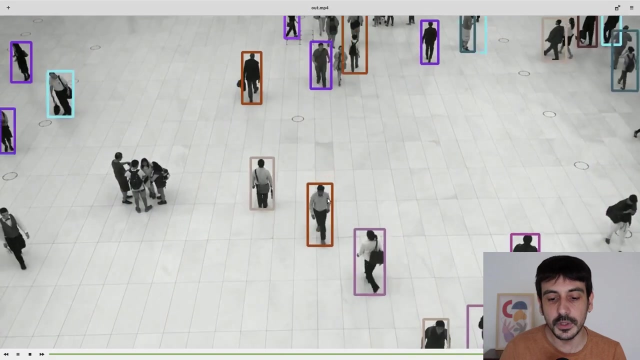 And the way it works is that as long as the object tracking algorithm, as long as DeepSort, is able to track each one of the persons in this video through all the different frames, then the bounding box will remain of the same color. If I show you an example, if you can see, this person over here has a brown bounding box and let's track all this person through all the different frames, you can see that the bounding box remains being brown through all the different frames in this video. 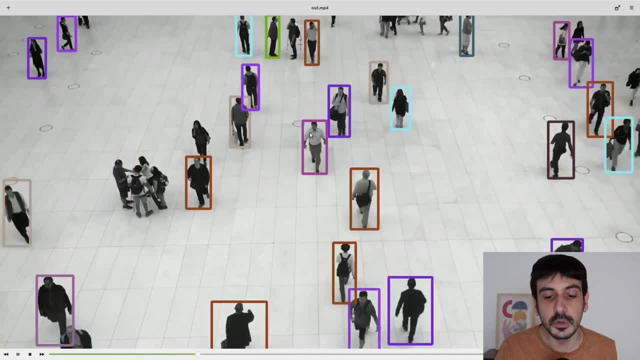 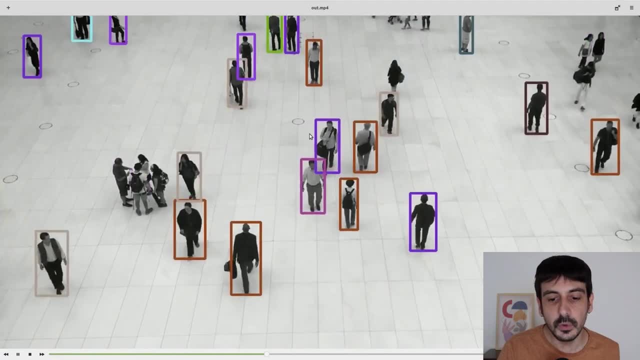 And I can show you another example, for example, with this person with a purple. You can see that this bounding box remains being purple through all the different frames, and the same happens with this blue bounding box over here, which means that the person is being tracked through all the different frames in this video. 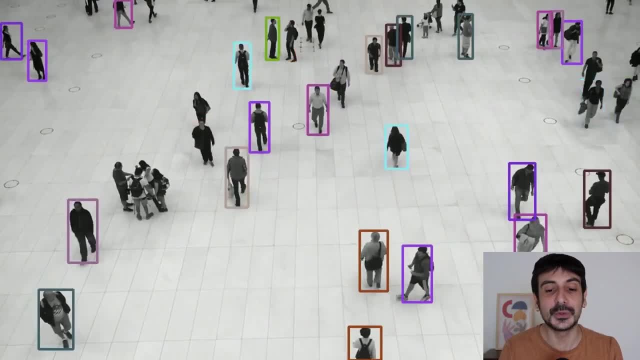 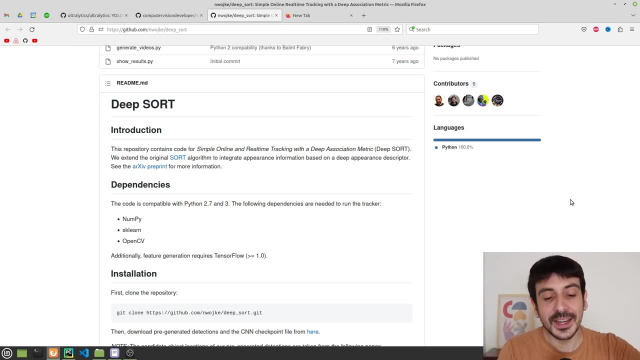 So this is exactly a project in which we will be working today, on today's tutorial, and now let's get started. So let's get started with this tutorial, Let's get started with this object tracking tutorial and let me show you the repository we are going to use in this project. 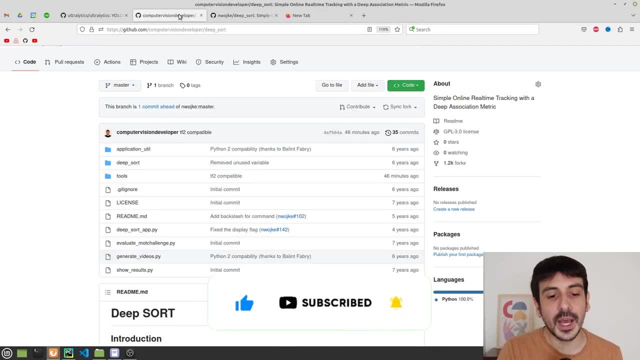 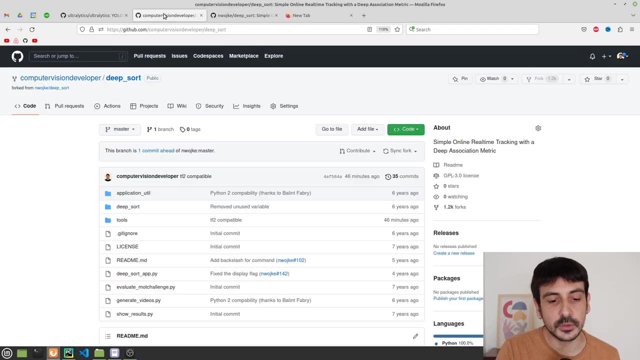 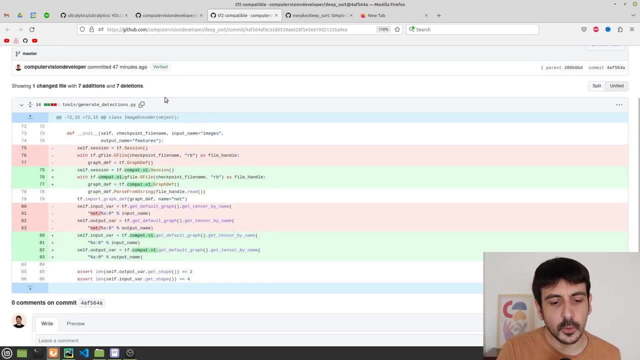 This is DeepSort official repository And we are going to Use a fork I made from this repository, which is this one. This is my account. This is a fork from the official DeepSort repository And the reason I made this fork is because I needed to make a change, a very small change, a very small edit, in one of the functions. 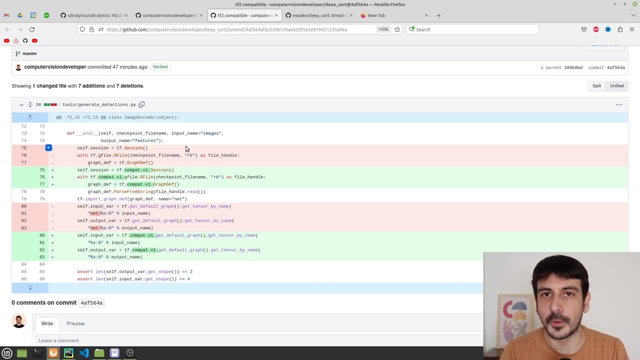 So I made this function TensorFlow2 compatible. right, I am going to use TensorFlow2 in this project and I need to make this very small change. But other than this, this is exactly the same repository of DeepSort. So this is the algorithm. 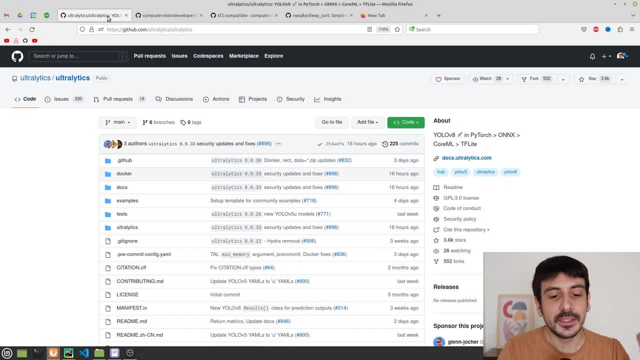 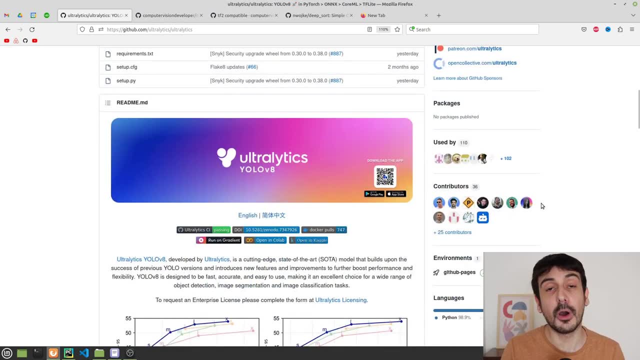 We are going to use in order to do object tracking. And now let me show you the object detector we are going to use in this project, because if we are going to track objects, if we are going to do object tracking, we definitely need data and we definitely need annotations. 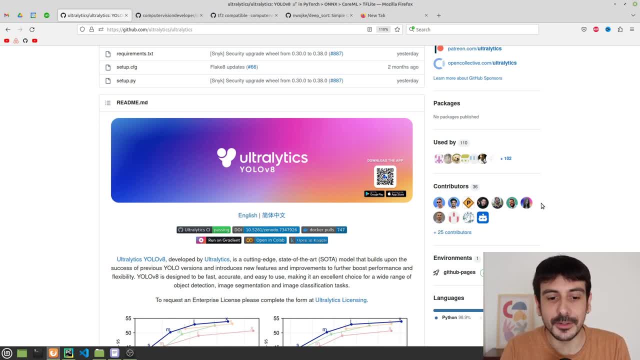 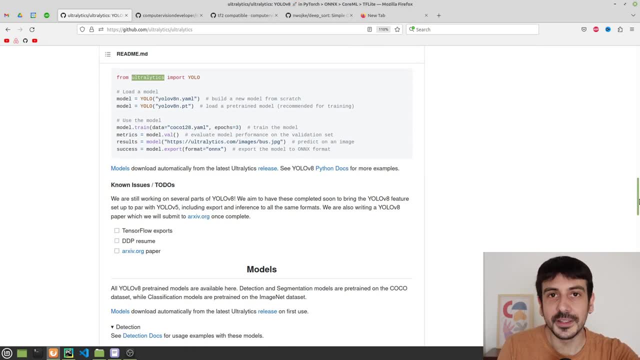 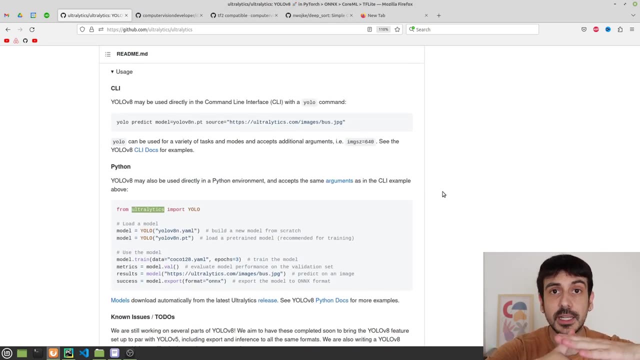 We definitely need detections on which to do some object tracking, Right? So this is exactly the algorithm, the object detector we are going to use in order to produce the detections we are going to input into DeepSort, Right? So we are going to use DeepSort as an object tracking algorithm and we are going to use YOLOv8 as an object detector. 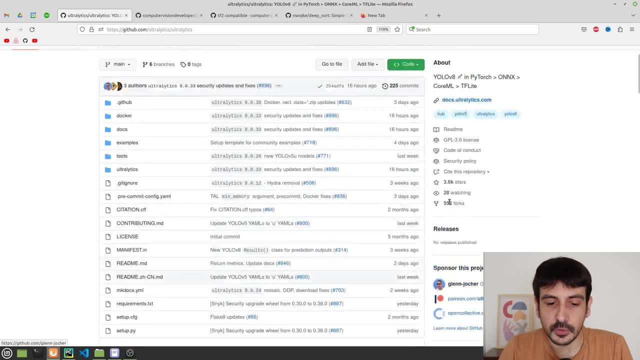 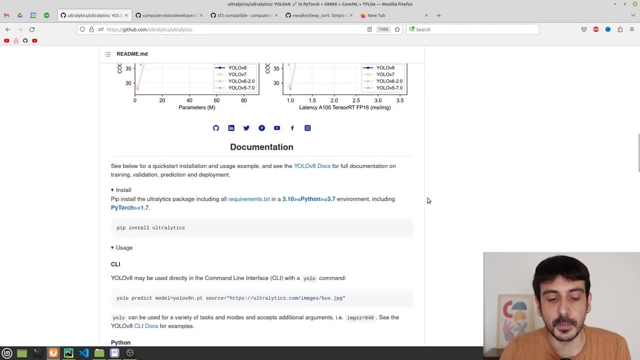 Right. So this is YOLOv8 official repository and we are not really going to use the repository itself, but we are going to call YOLOv8 through a Python package. YOLOv8 is available through a Python package. 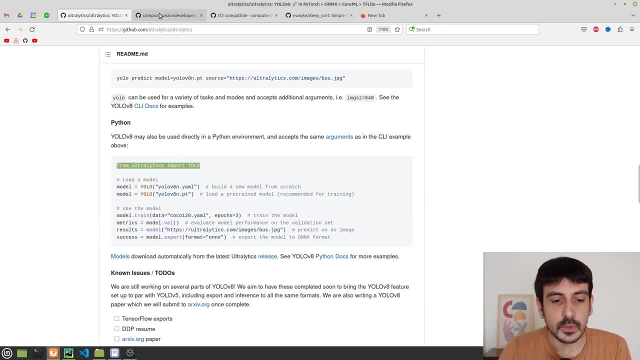 So this is exactly how we are going to use it, But this is only to show you how the YOLOv8 official repository looks like, And I'm going to post a link to this repository In the description of this video. So now let's continue. 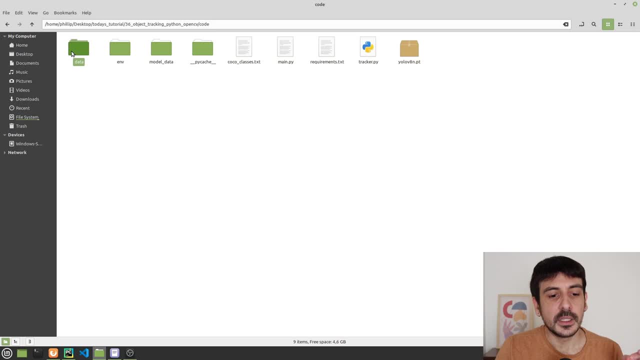 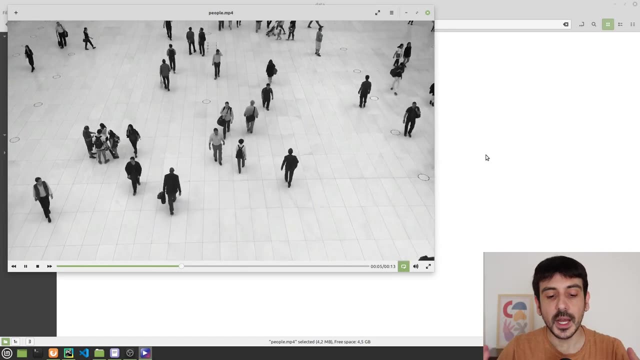 And now let me show you the data we are going to use in this project. This is a video we are going to use in order to test how the object detection works and how the object tracking works, And you are probably familiar with this video. 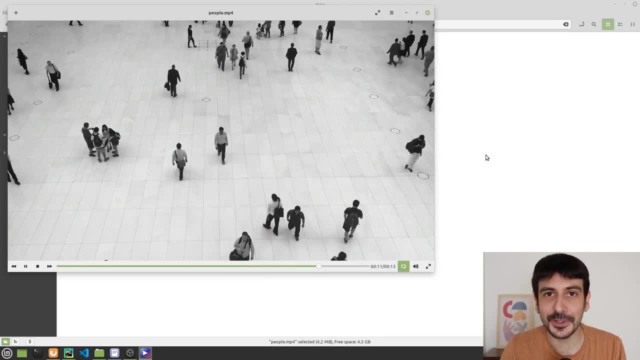 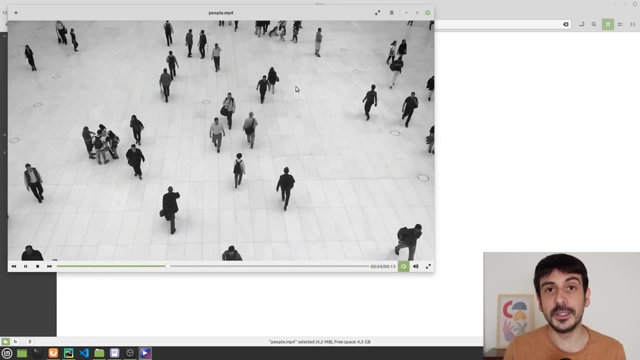 This is a video which is very commonly used in this type of tutorials on object tracking Right, So you are probably familiar with this video already And you can see that this is a video of many, many, many people who were just walking around. Right, So you are probably familiar with this video already, And you can see that this is a video of many, many, many people who were just walking around, Right, So you are probably familiar with this video already, And you can see that this is a video of many, many, many people who were just walking around. 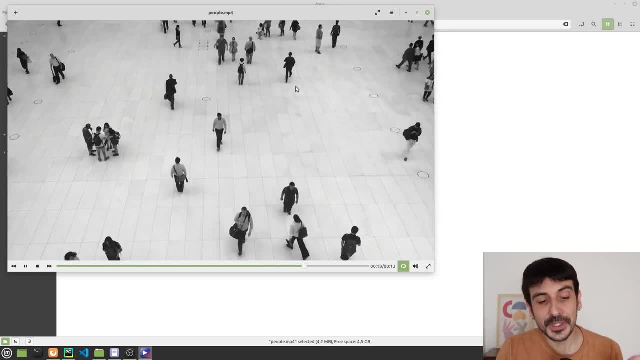 Right. So you are probably familiar with this video already And you can see that this is a video of many, many, many, many people who were just walking around One place to another and so on. So we are going to use this video in order to test everything. we're going to do one to this tutorial. 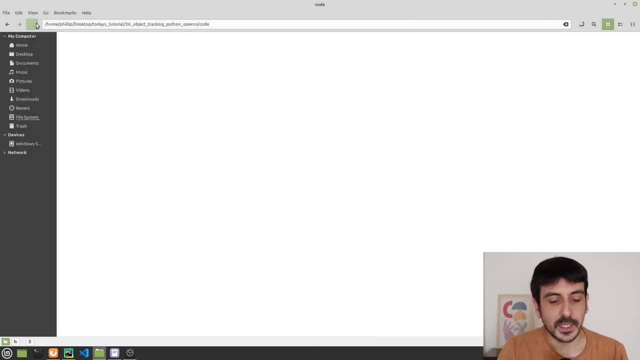 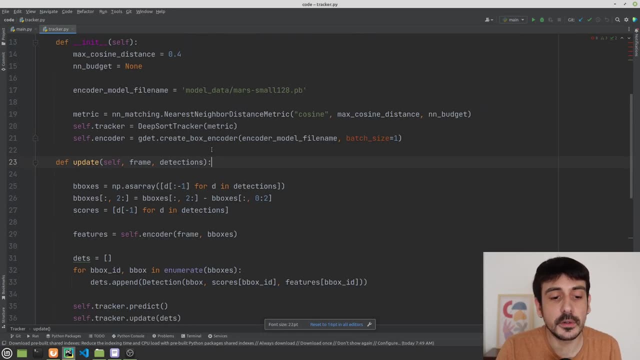 So this is the video- is the data we are going to use today. Now let's go to PyCharm, because I need to show you a file I have created. This is something like an auxiliary file I have created which is going to make things much, much, much simpler on this tutorial. 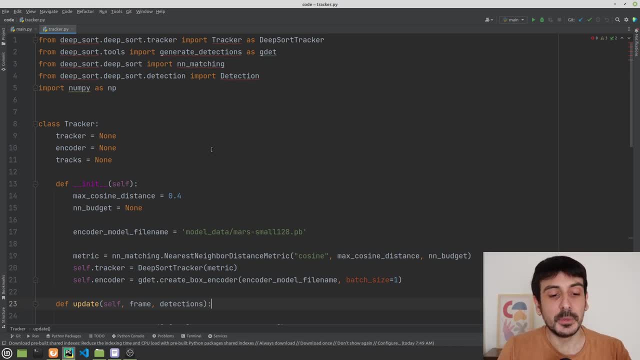 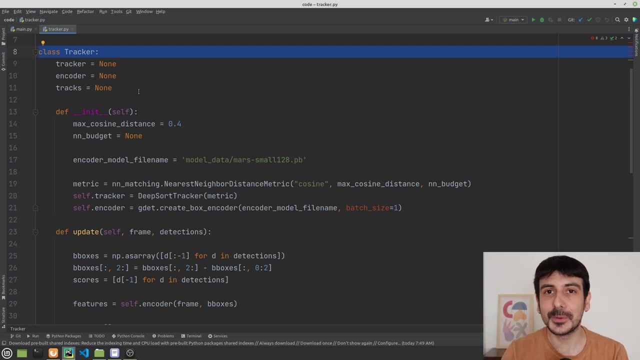 It is going to help us a lot on everything we are going to do today, because this file file, it's called trackerpi and it contains a class which is called tracker, and this tracker is basically a wrapper around deep sort. right, we are going to use deep sort, but we are going to use 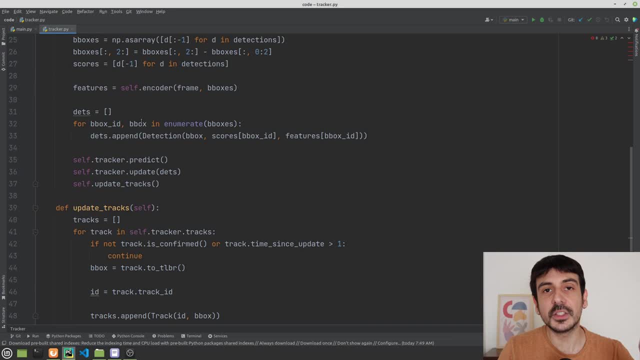 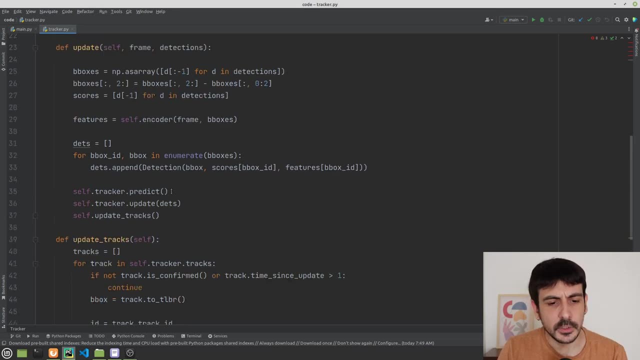 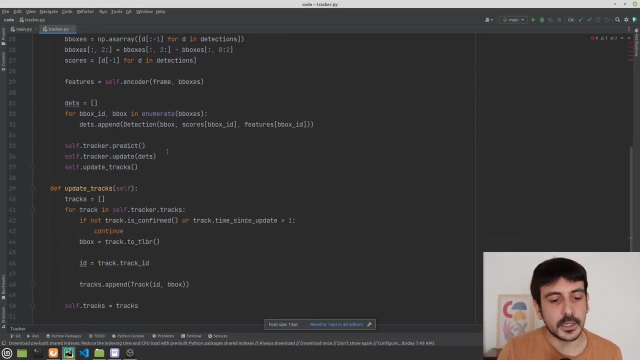 it through a wrapper I created in order to make things much, much simpler, in order to make all the process much more straightforward and much, much better. you can see that this wrapper has a few functions, and the idea of these functions is to just grab all the complexity and all the different. 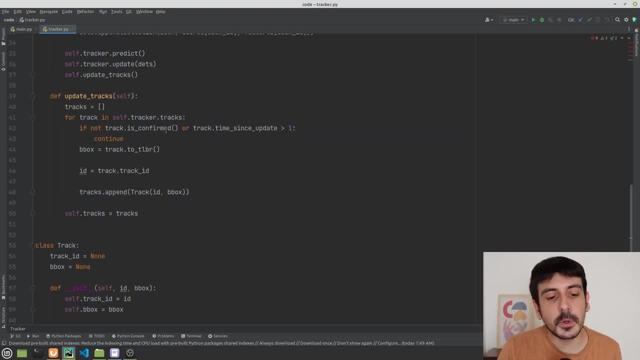 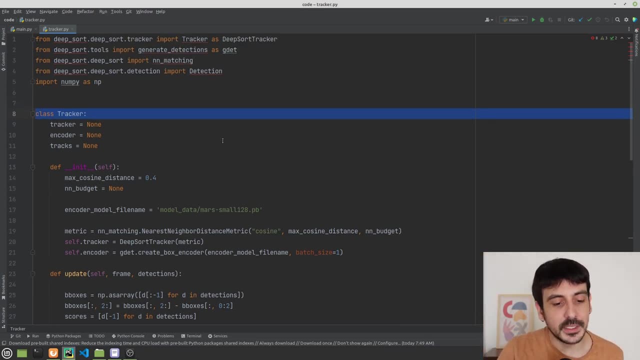 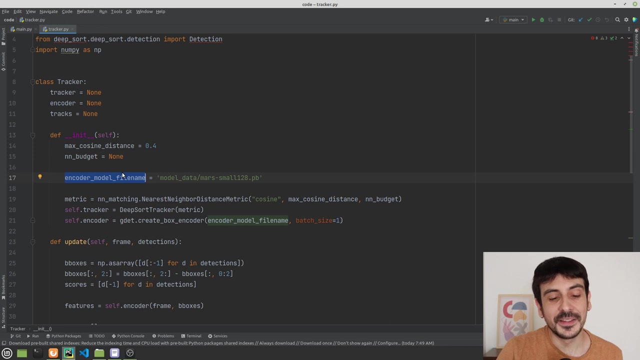 details of how to use deep sort, so we don't really have to mind about all this complexity and we can just use deep sort from a very, very high level using this wrapper. right, and a very, very small detail regarding this wrapper is that you can see, I have hard coded this path, which is the path to: 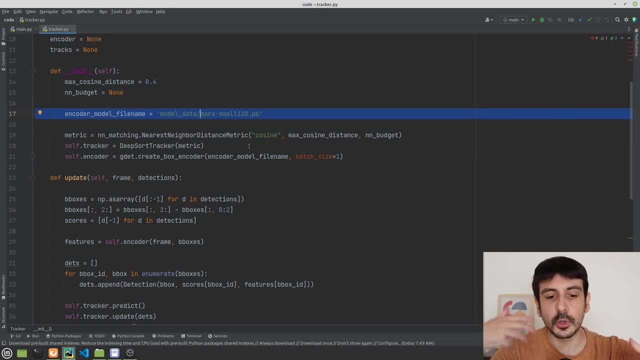 a model with which deep sort needs in order to compute all the process and so on. right, in order to compute all the object tracking. this is a file, this is a path I have hard coded into this grapper, so please remember to download this file, which I'm 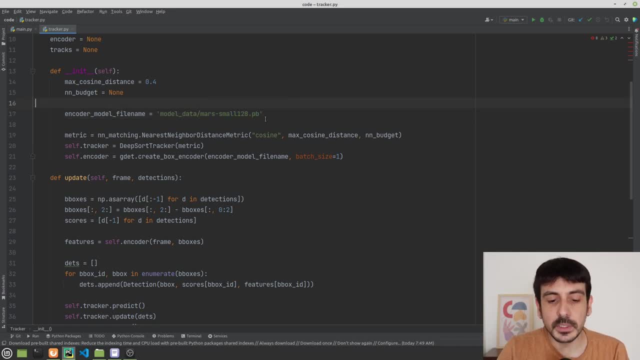 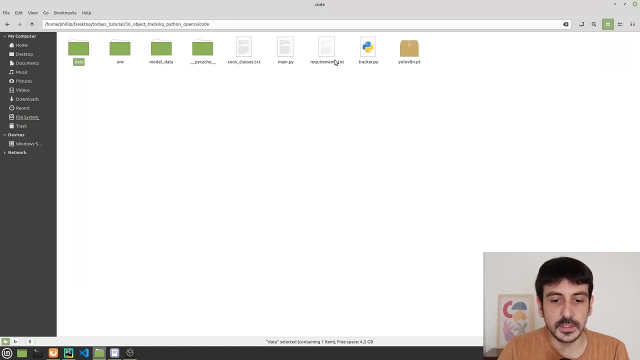 going to tell you exactly where it is in the description of this video, and please remember to save this file in exactly this location, right? if I show you my root directory, which is this one, you can see that I have created a directory which is called model data and inside model data I have 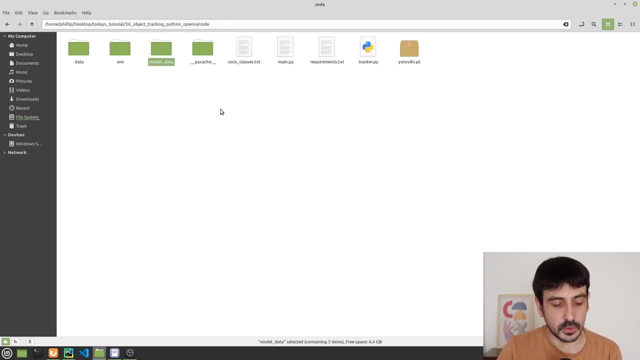 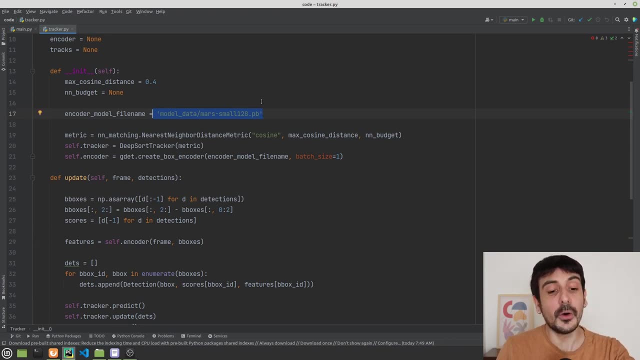 these three files, right? please remember to follow the same structure, because otherwise this is not going to work, because this is hardcoded, right? so please remember to do that, or please remember to edit this line so you can specify the location, the path to the model, right, because you definitely. 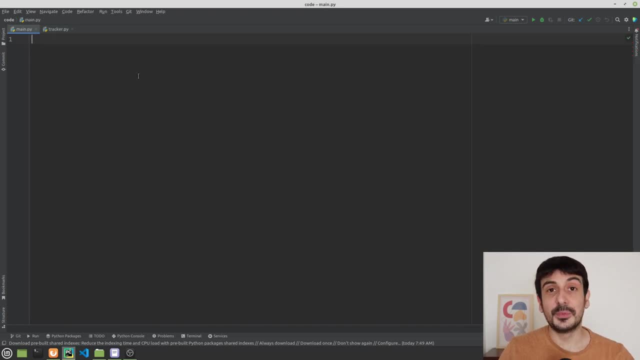 need this model in order to run this iron. so that's pretty much all you need to know about the repository we're going to use, about the algorithm we are going to use, about the object detector we are to use, the data, the video we're going to use in order to test the performance of the of today's 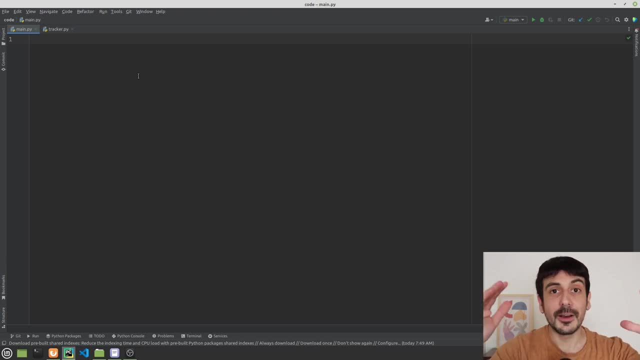 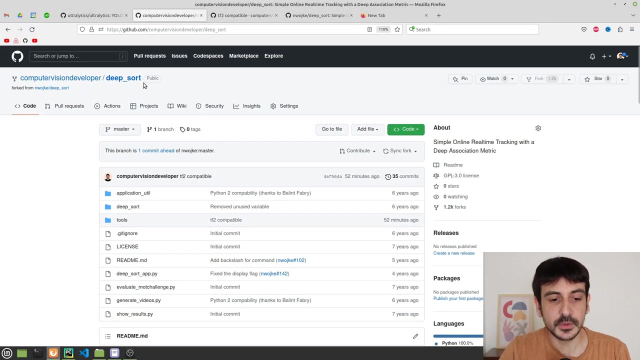 tutorial and this wrapper i have created, right. i have already showed you all these details and now we can just start with our tutorial. we can start with our coding, right. so the first thing we're going to do is to clone this repository, this repository, deep source repository, but we're 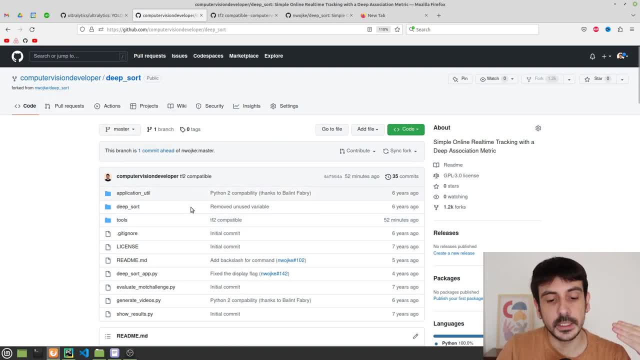 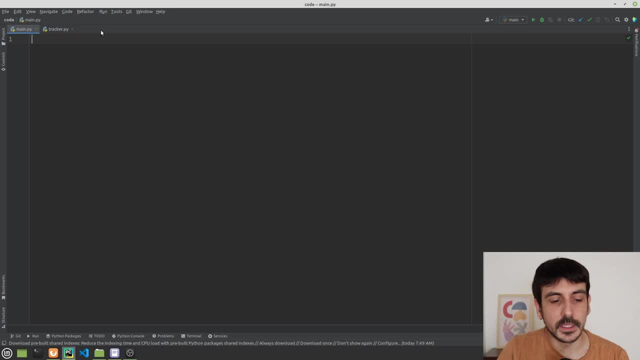 going to clone my fork, the repository i have forked and the changes i have made. otherwise it's not going to work. otherwise it's not going to be compatible with all the dependencies i have specified for this project. let me show you super quickly the requirements file and you can see that. 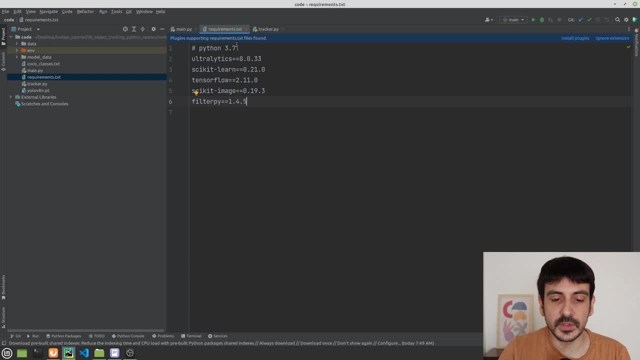 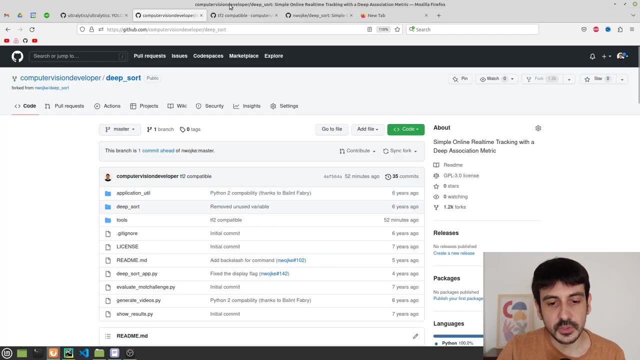 i have also specified the python version i'm using, which is three python 3.7, and this requirement, which is tensorflow 2.11. we need to make these, uh, small changes. i show you over here in order to make these changes, in order to make these changes, in order to make these changes, in order to make. 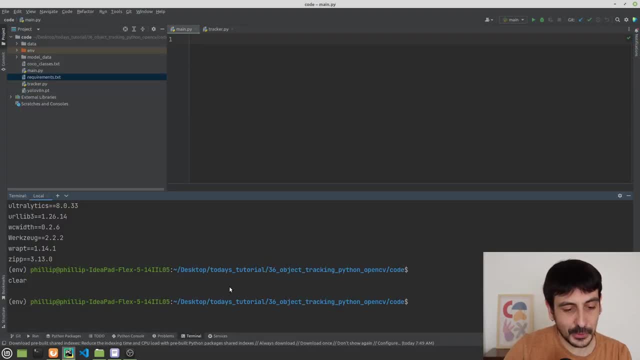 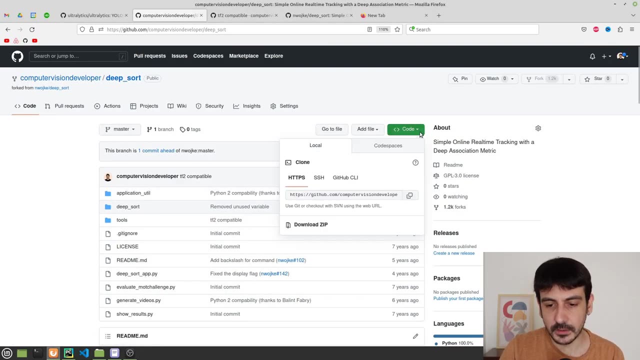 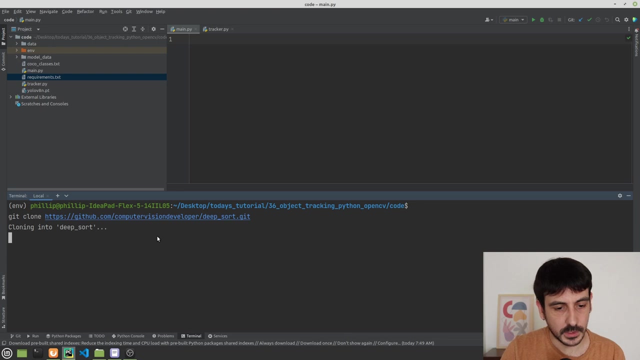 this compatible with this tensorflow version. so now we're going to clone the deep sort repository i have forked. so we're going to clone the, the one that's in my account, and i'm going to copy the url: git clone and that's pretty much all. so i have cloned this repository and this is. 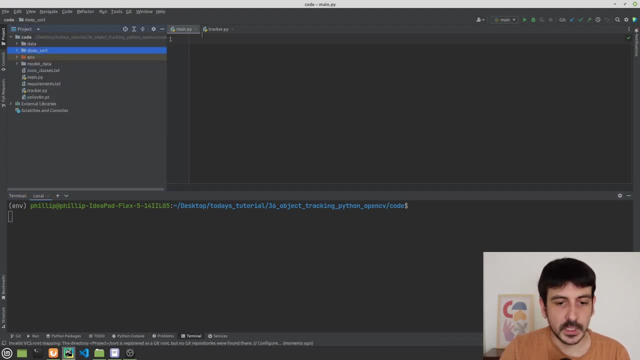 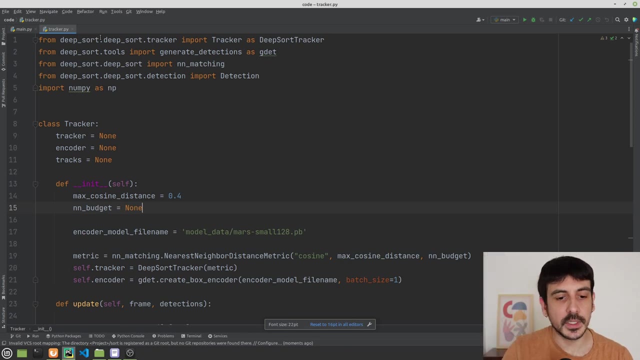 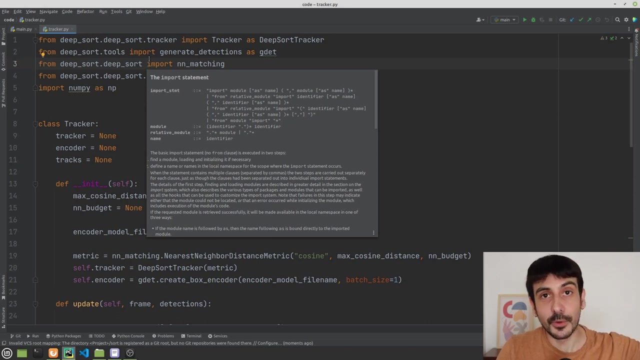 if i refresh, this is where the repository has been cloned, because you can notice that if i go back to trackerpi, at the top of this file, you can see that there are a few imports which are in, which is importing files from deepsort. now this is not going to work unless you clone. 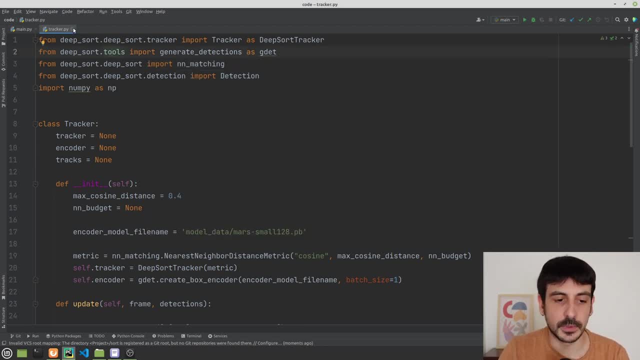 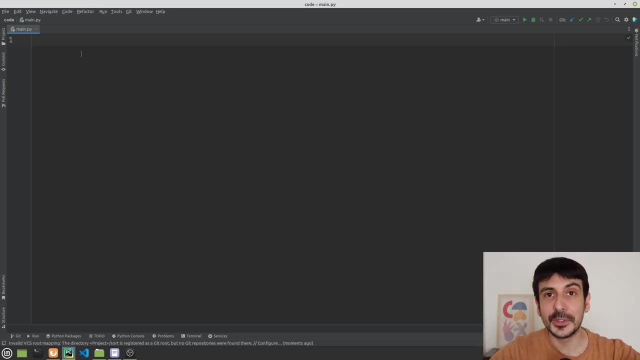 deepsort repository. so please remember to do it as a first step. so that's pretty much all i, assuming that you have already installed all the requirements, that you have already cloned deepsort, that everything is just completely ready and you can just start working on this project. 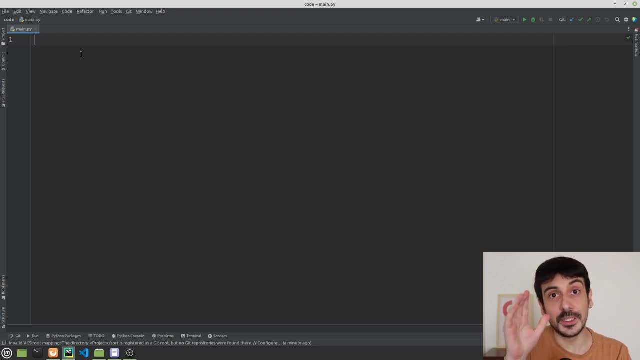 this is how we're going to do. we're going to take it one step at a time. it's always a good idea to take projects one step at a time. so let's start by importing os and by importing opencv. now let's define the location, the path to the video we are going to use and in order to move, 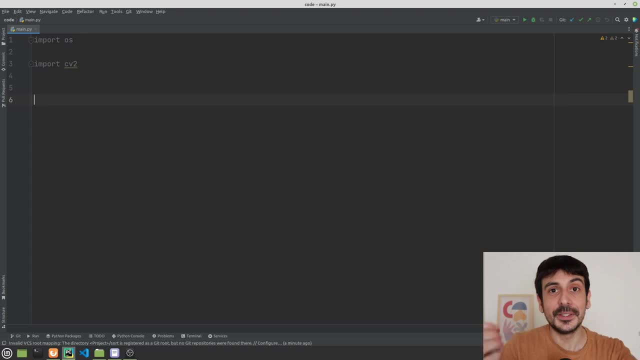 once by time. the only thing i'm going to do for now is just reading this video, loading this video, and i'm going to display one frame at a time. right, i'm going to display using him. show one frame at a time so we make sure we can read the video and we can visualize the frames in this video. 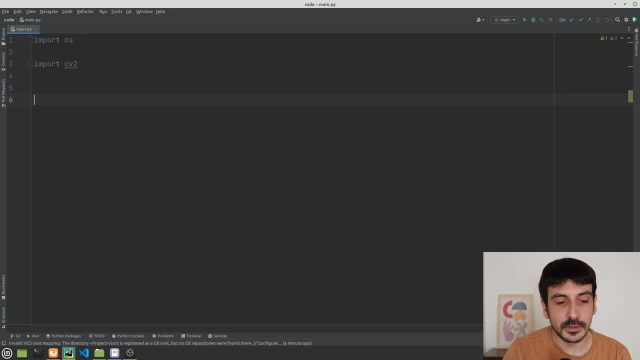 that's going to. that's what i'm going to do in order to get started on this project. so the video path is seen as part join data and the video is called peoplemp4, which is a very appropriate name for this video because it contains people. right, it contains people walking, so it should be. 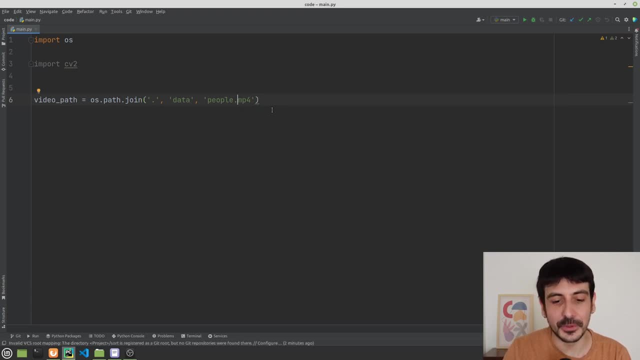 something like people walking dot mp4, but people mp4 is. it's just fine. so now I'm going to call cvchew dot video capture and I'm going to specify this video location, which is here, and this will be called cap. right, let's take it. 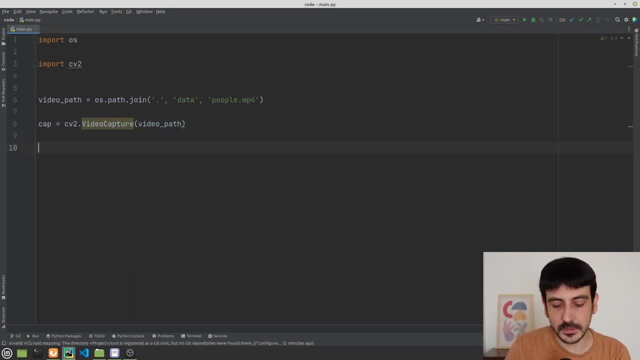 one step at a time. now what I'm going to do is I'm going to read a frame from this video. so cap dot read. this will be read frame and no while read. I'm just going to visualize frames from this video. so CV to im show this window will. 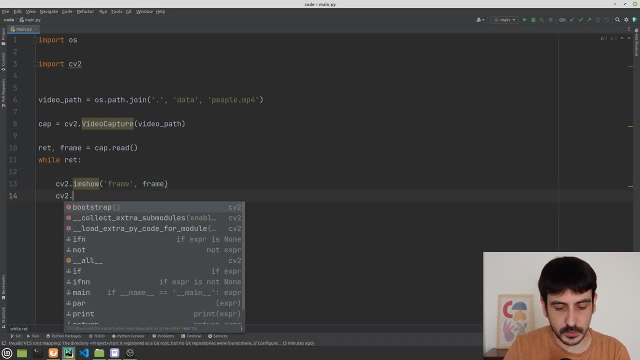 be called frame. I'm going to specify something like 25ms will be just fine, And obviously I have to read a new frame, so redframe equal to capread. and I'm going to release the memory before I forget, and I'm going to destroy all windows by calling. 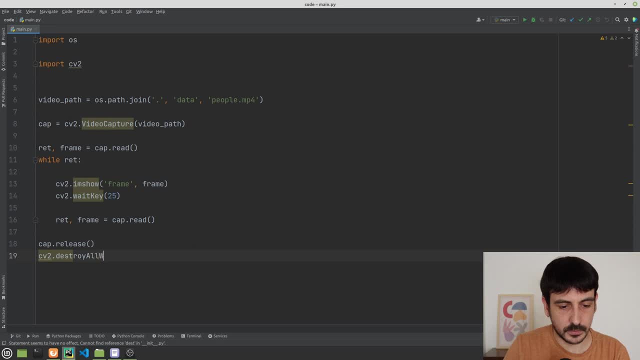 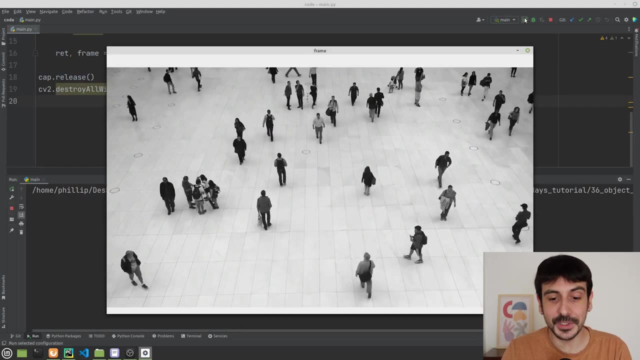 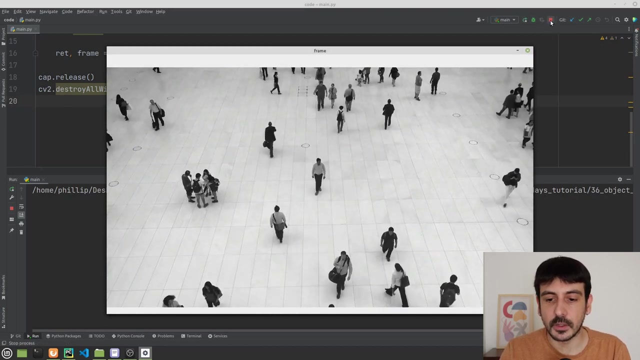 this command. Ok, so that's pretty much all. So let's see if we can execute this piece of code successfully. Let's see what happens. and you can see that we are just looking at the exact same video I showed you a few seconds ago. 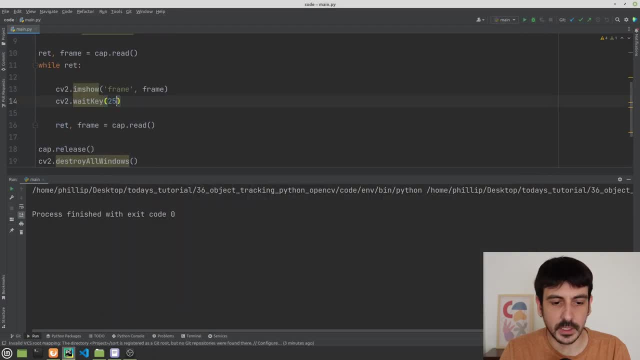 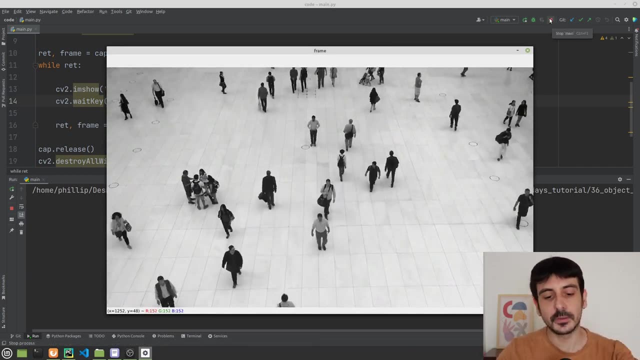 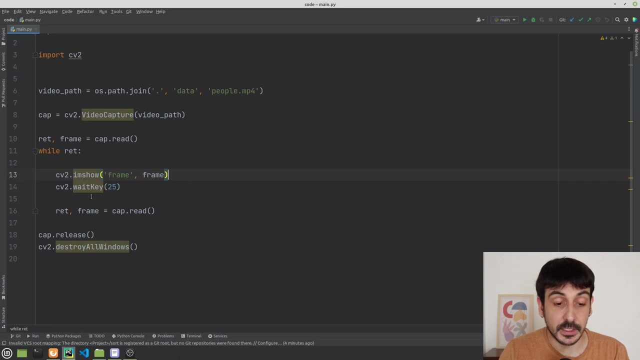 We may need to adjust these 25ms because I have the impression it's running a little faster than in the original video, but it doesn't matter. this is only to show you that we can successfully execute this. We can read this video and we can just display one frame at every time, at every execution. 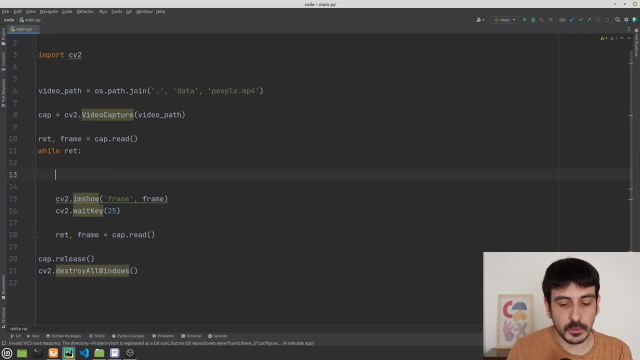 And now let's continue So we can read frames from this video. we are reading frames and what we need to do now is to use YOLOviate in order to produce our detections- right, The detections we are going to use in order to input these detections into the object. 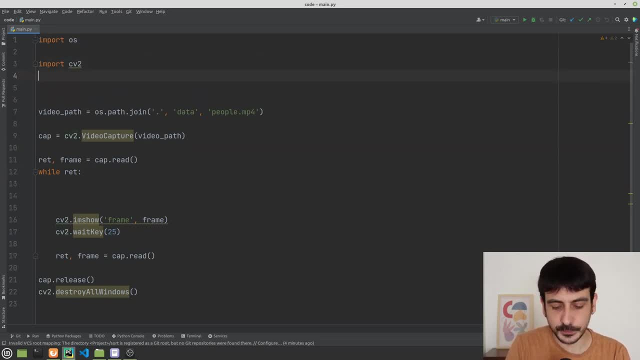 tracking algorithm In order to do that. I'm going to import from Ultralytics, import YOLOviate And I'm going to do something like that. I'm going to define it somewhere around here, Maybe somewhere around here, And I'm going to say: model will be YOLO and I'm going to specify the YOLO model. I'm going 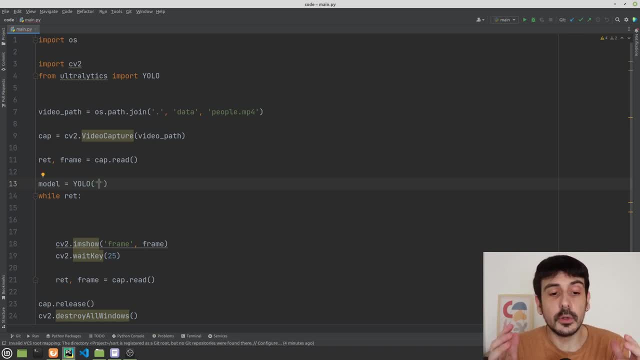 to load, And I'm going to work with the YOLOviate pre-trained model. right, You can just use a pre-trained model from YOLOviate in case you don't have a model already. so that's what I'm going to do. 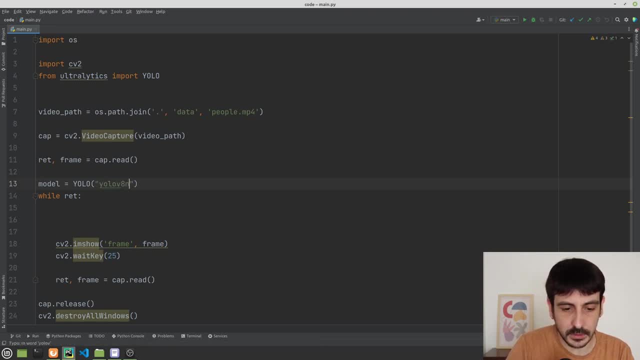 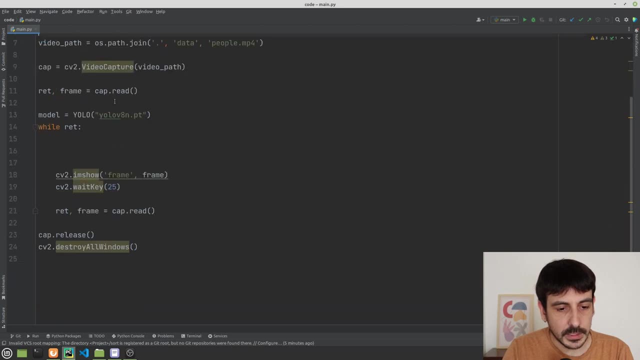 Now. so the model is called YOLOviateNanopt, if I'm not mistaken, and this is exactly the model we are going to use. So let's take it one step at a time and let's see if we can just execute this code. 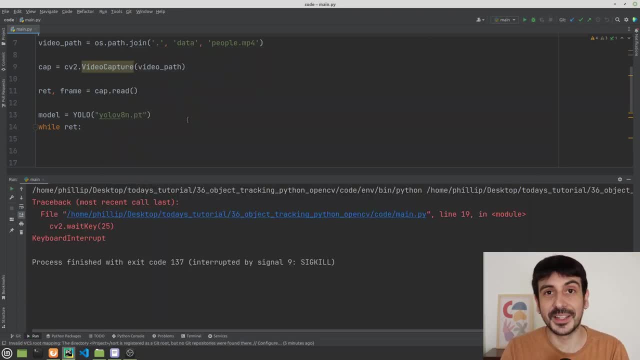 Let's see if we can just create the model. Everything seems to be working fine because we didn't have any error. So now let's continue. Now let's produce our detections, and in order to do that, I am going to call model dot. I'm 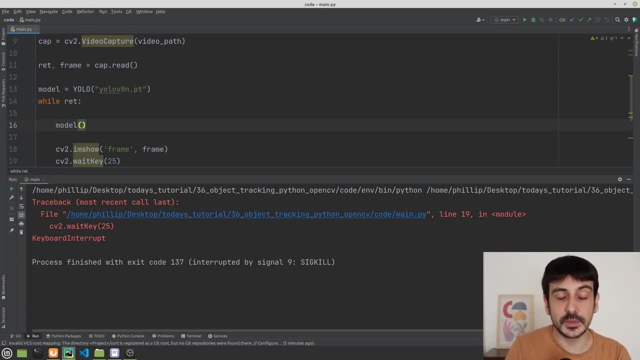 going to call model and I'm just going to open these parentheses, because this is something like a function we are using, and I'm going to input the frame I have just read from the video. right, I'm just going to input this frame and I'm going to call the output detections. 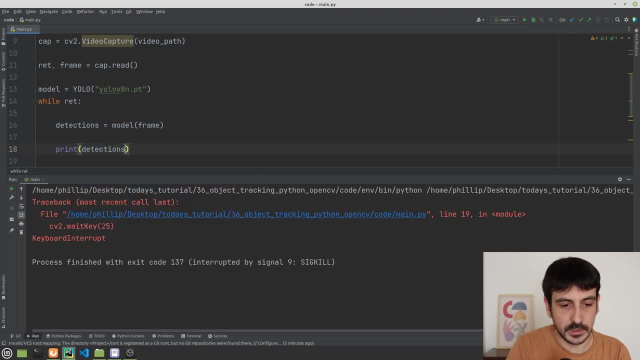 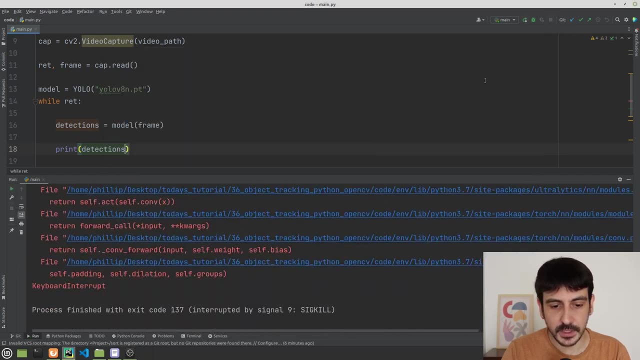 In order to go one step at a time. again, I'm just going to print detections and let's see what happens. Okay, You can see that I am getting something. I'm getting a lot, a lot, a lot of information. 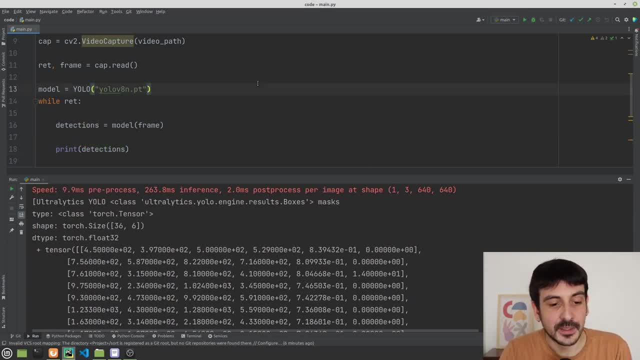 So everything seems to be working just fine. So we are moving one step at a time, but you can see that we are making a lot of progress, a lot of progress. So now what we need to do is to unwrap these detections, right. 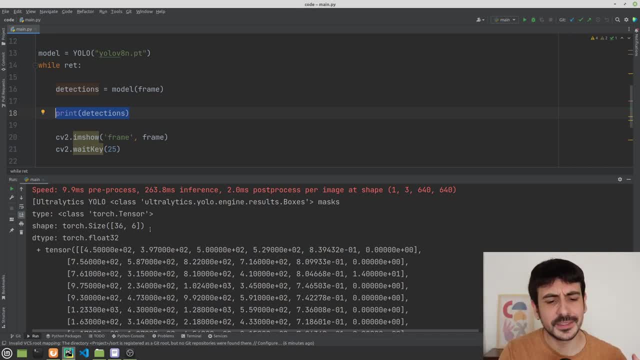 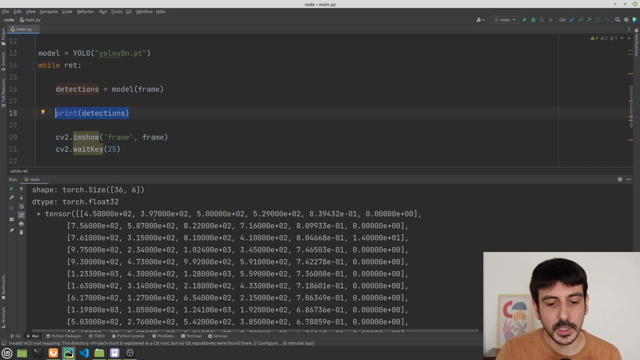 Because we had something which looks like this: it's like an entire class. This is something that it contains absolutely all the information we need in order to work on this tutorial, In order to get the tracking and so on, But this may not be in the exact format we need it to be. 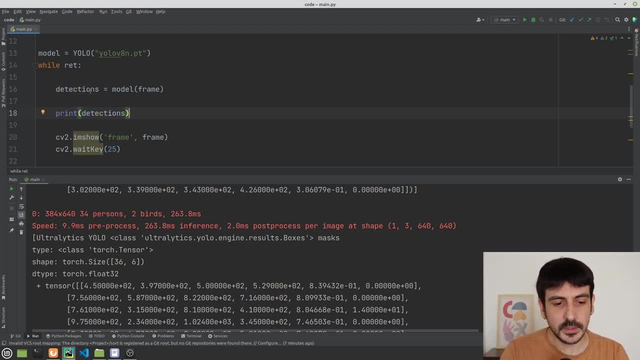 So we need to unwrap all the information from here. I think it's better to call it results instead of detections, because I'm going to use detections later on, So maybe I can just use results. Okay, So results give results is a list containing all the detections. 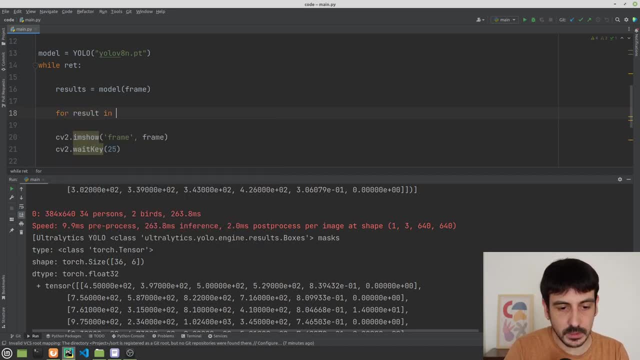 I am going to something like this: I'm going to iterate for result in results, And as I am- Yeah, As I am making the inference of a single frame, of an individual frame, this will always be a list of length one. So, doing like this, we are doing this. 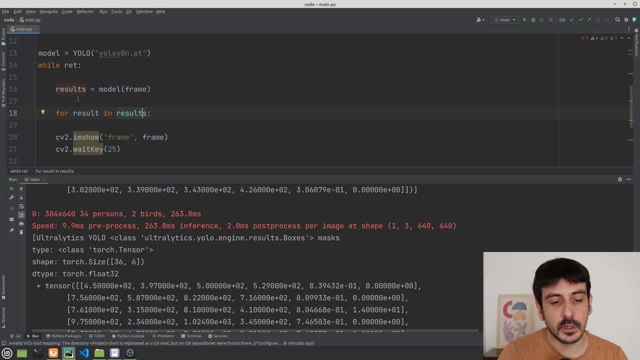 We are iterating in a list of length one long story short. we are doing this iteration, but actually we are only doing one iteration right, There's only one object inside results, So we are just doing these four ones. We could do it in a different way. 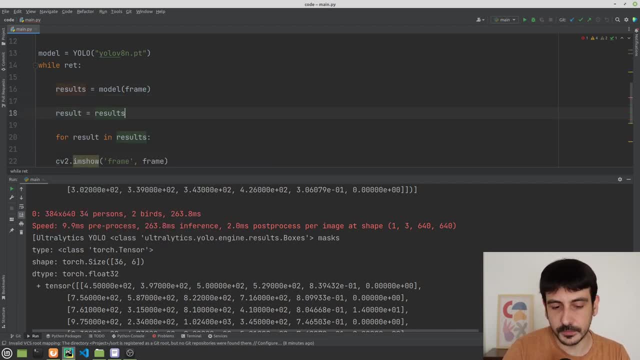 We could do it like results equal, results zero. We could do it like this too, But I think it's a little cleaner if we just do this iteration. but remember, we are doing this process only once. we are doing this duration only once, because there is only one object. 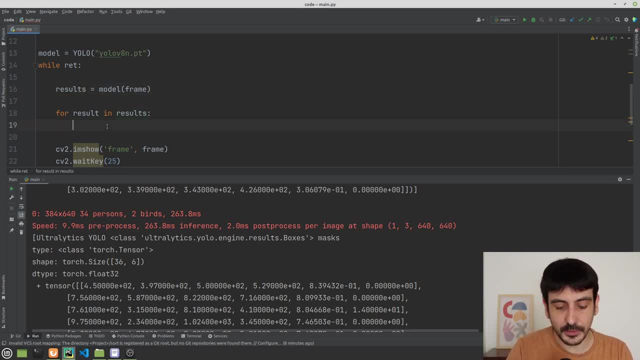 inside results. And now let's call another object, another list, which is called detections. This is where we are going to save all of our detections. And now let's do something like this for our in results dot boxes. Uh, I think this was something like. 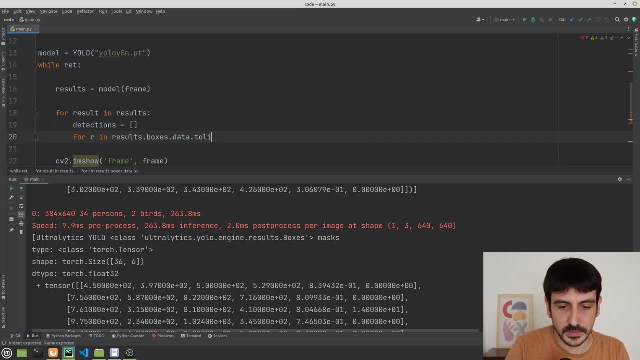 Boxes, dots, data dots, to list something like this, because this is like a very, very custom object type in um in Yolo V8 and we need to make it to look something like a list. We can, we, we need to be able to iterate in, in in this object. 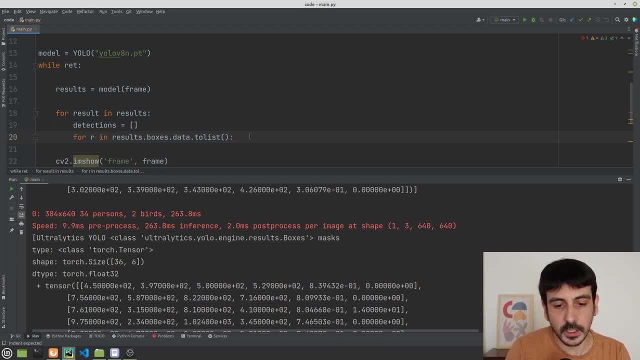 And I think this is the way to do it. If this is not the way to do it, we are going to get an error and I can just um fix it. And once we are iterating in this object, we are going to do something like this: 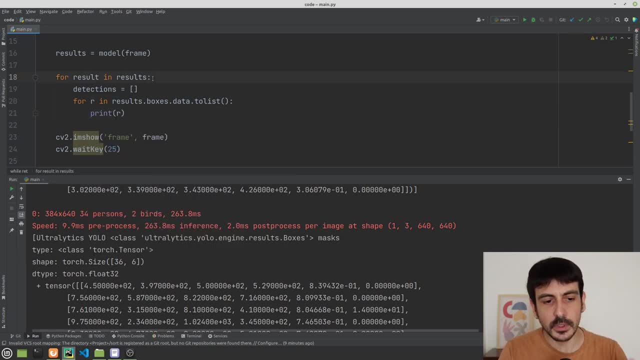 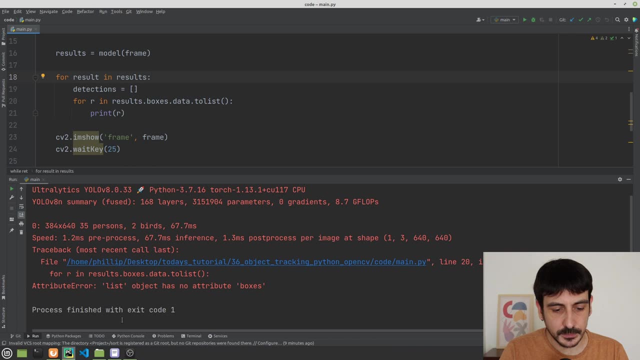 We're going to print it To see if it works, To see how it looks like, And then we are going to un-grab all the information from within this object. Let's see. No, I had. I've made a mistake. 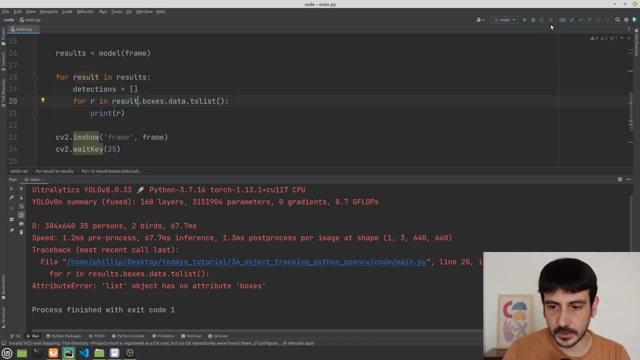 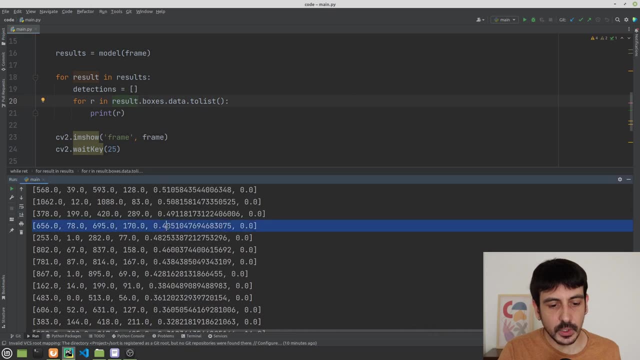 All right, Because I'm iterating here and actually it's here. Now everything should be okay. Everything's okay And this is the results we are getting right. This is our, this is the print we are doing over here, And you can see that this is exactly how it looks like. 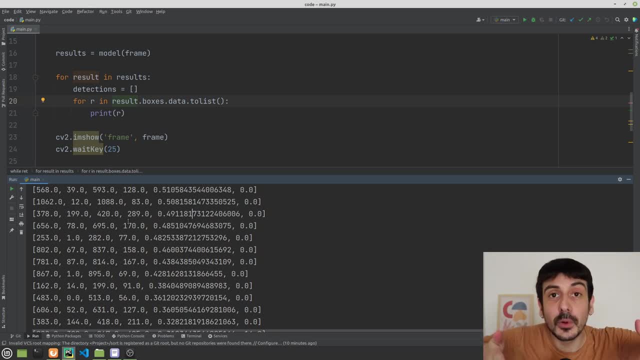 And this is all the information we need from more detections. right, This is all the people we are detecting in this video, And the way we are going to un-grab this information is like this: We're going to say: this is X1, Y1, X2, Y2, and then confidence value. I'm just going. 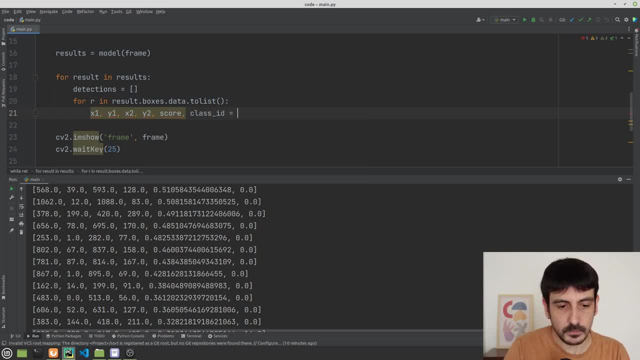 to call it score and class ID. This will be R right. Remember that we are using a pre-trained model from YOLOv8 and this model was trained on the COCO dataset, So we are detecting All the COCO classes. 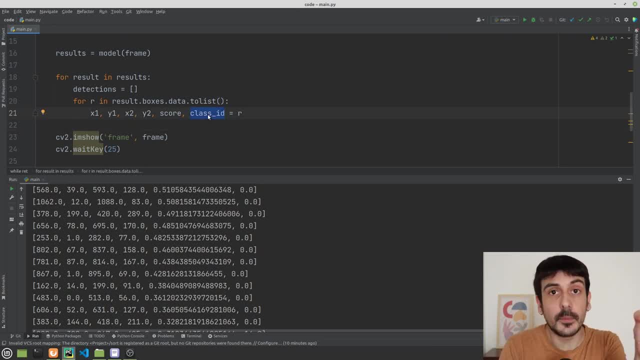 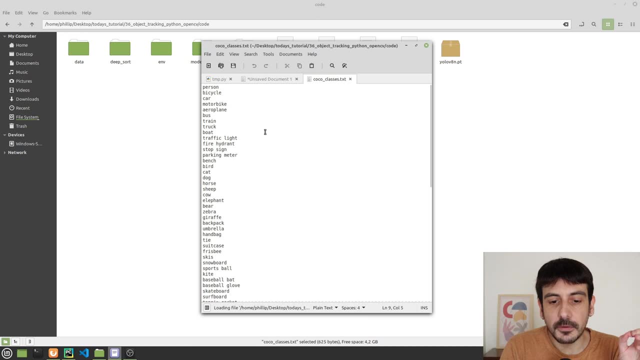 So we are going to have a class ID which is exactly the class we have detected in this dataset. If I show you my local directory, my root directory, this is a file containing all the classes we are able to detect with this model. 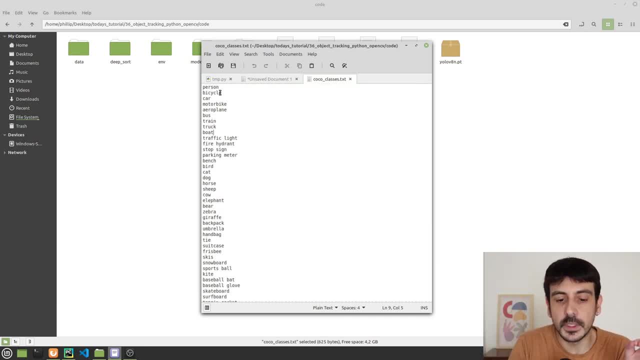 And this also tells us the index for each one of these classes. in the case of person, which is the object we are going to detect more more often in this video, this is the first element in the list, which means it's the class ID: zero, right. 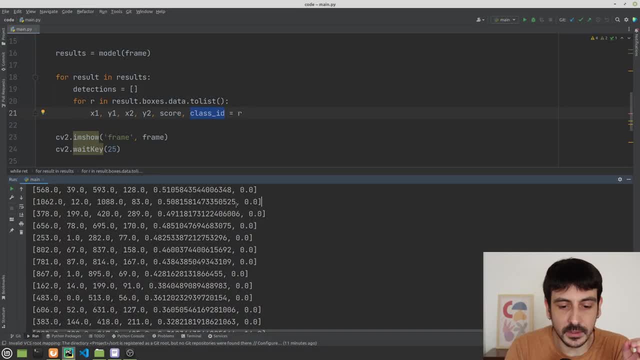 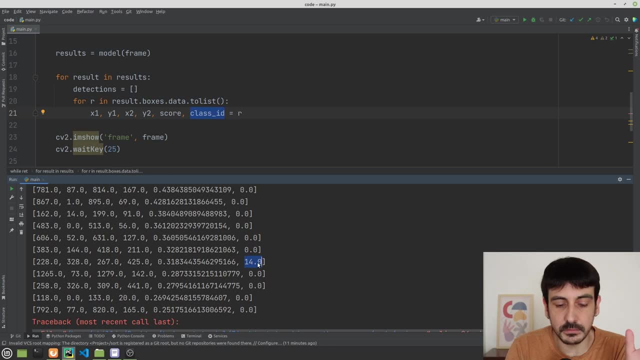 It's the index zero And if I go back, you can see that this number is always zero for absolutely all detections. Now we have detected something different than zero. This is 14.. Maybe it's another object, but you can see that in most cases it's a zero. 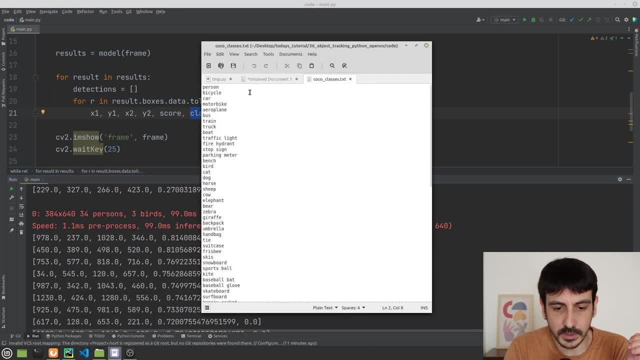 We're also detecting a 14.. We're also detecting a 14.. Let's see what is 14.. This is zero. So 14 is birth. We're detecting birth. We're detecting birth in this video. Maybe, I don't know. 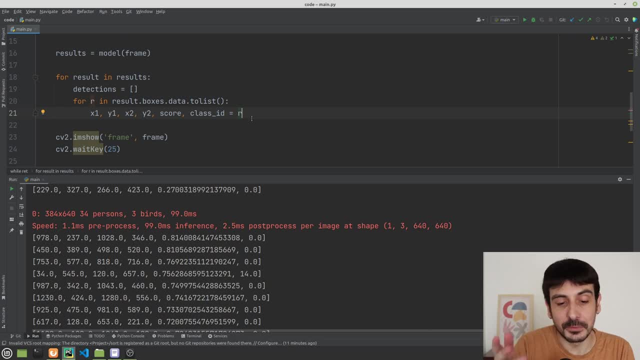 I don't know what's going on. Maybe we're detecting this birth with a very low confidence, or maybe there are births I haven't noticed, or maybe it's a misdetection and it doesn't matter. Now let's continue. So these are the detections we are getting. 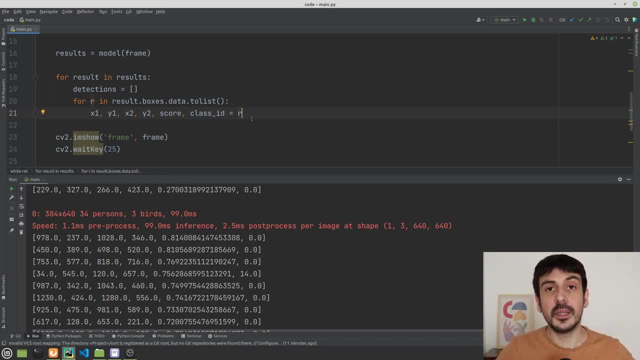 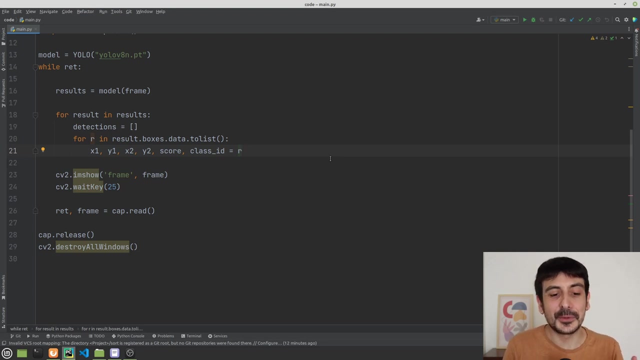 We are unwrapping all these detections and now it's a time to call our wrapper. right Now that we have successfully unwrapped absolutely all the detections from YOLOv8, from this YOLOv8 object, Now it's a time to call DeepSort object tracking in order to start doing our tracking. 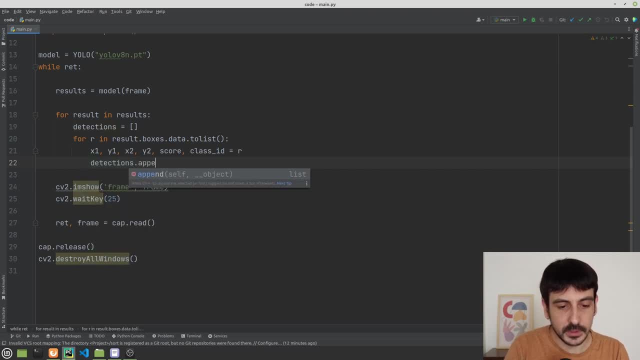 And I'm going to do something. I'm going to detectionsappend and I'm going to create a list which is X1.. I'm just going to call, I'm just going to save all of this right. This is all the information DeepSort needs in order to do the tracking. 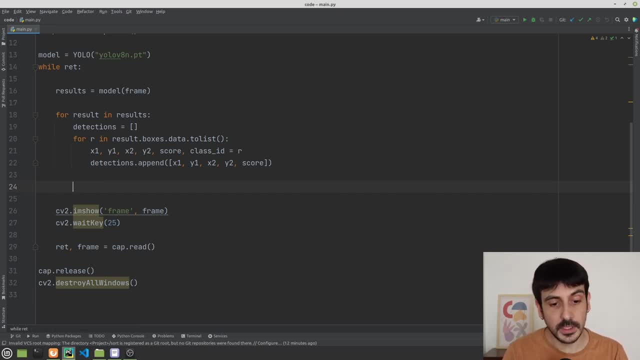 And now we have the detections, The only thing we need to do- Yeah, The only thing we need to do- is to call the tracker. Maybe I can do it as an integer, otherwise I may have a problem, or maybe another way to do it. 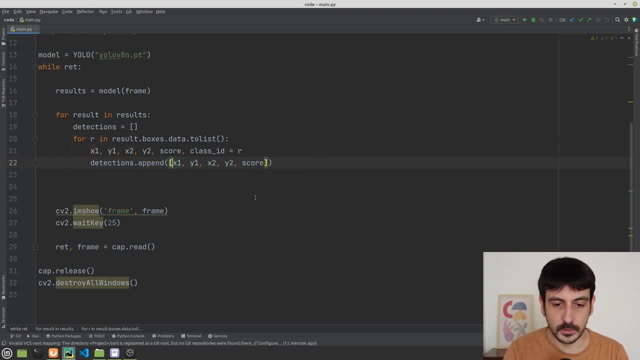 Maybe another way to do it is do it here, So we just read everything as a integers. let's say X1 equal to int X1, and let's do exactly the same for all All the other variables. these are little noisy, but it's okay. 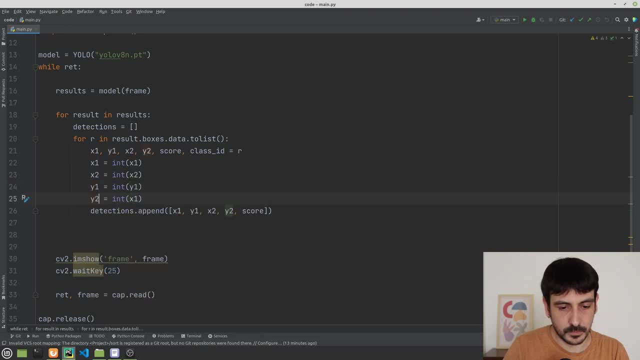 Okay, And this is the same with class ID. Okay, Okay, Everything's okay. Okay, so we have unwrapped all these objects and we have converted everything into integer, or everything that's an integer. we have made it an integer and now it's a time to call the wrapper in order to 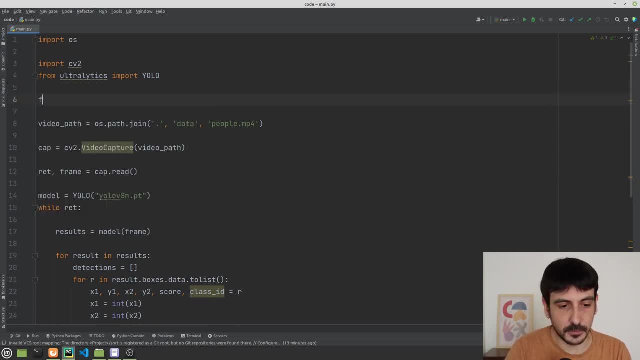 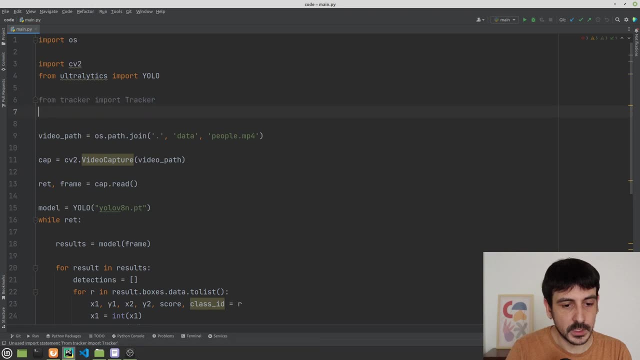 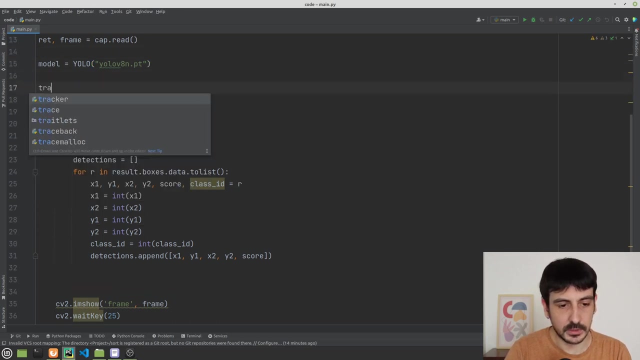 do that. i'm going to import the wrapper first, which is from tracker import, import tracker. and now that we have imported the tracker, the only thing we need to do is to initialize it. i'm going to do it here: tracker equal tracker. i'm going to create a new instance. 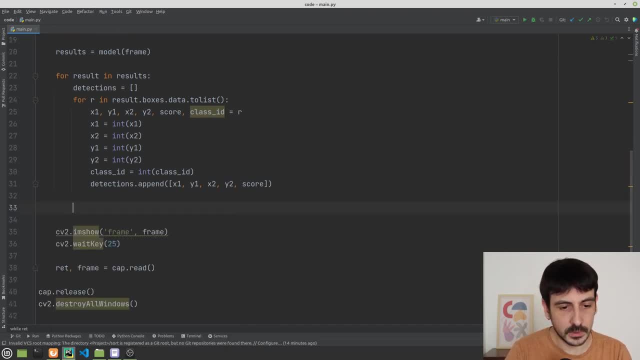 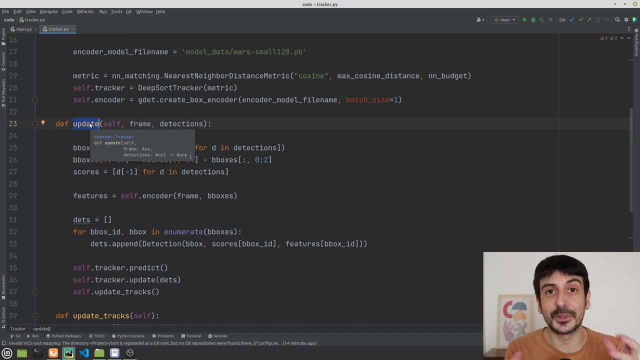 and then the only thing we need to do is to call- i'm going to do it here- tracker dot update and we need to input. let me show you what we need to input in order to call update, which is the most important function of the tracker, because it's where it's going to update all. 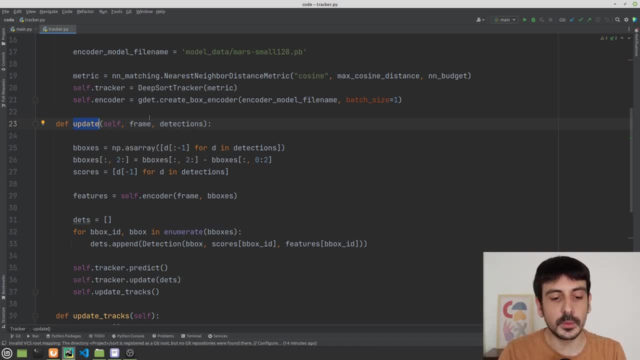 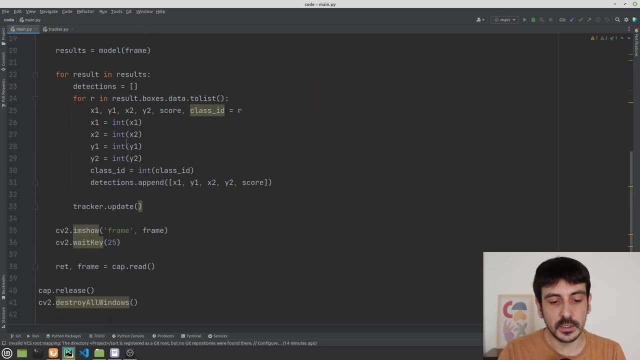 the tracking information and everything that's going on in this video. we need to input two parameters, which are the frame and the detections. right, and so the detections: we have just created, exactly the same object we have created over here, and then we also need to input the frame. 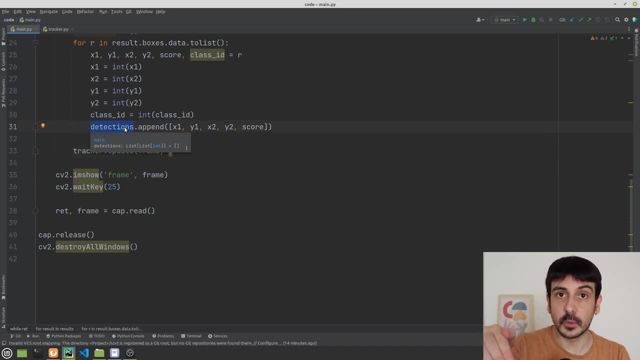 remember for the way object tracking works, for the way deep sort works, for the way this specific algorithm works, the. the algorithm computes some features on top of the frame, on top of the um, on top of the objects which were detected. right, it's going to crop the frame and it's going 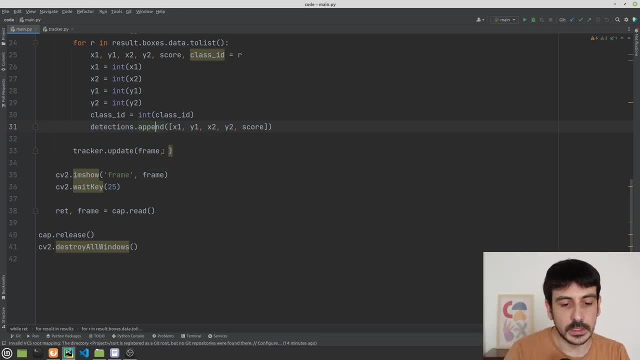 to extract some features from it. so we need- we definitely need- to input the frame and then detections. okay, and now the only thing we need to do is to iterate in all the tracks in this iron. so we- i'm just going to call for track in trackertracks. 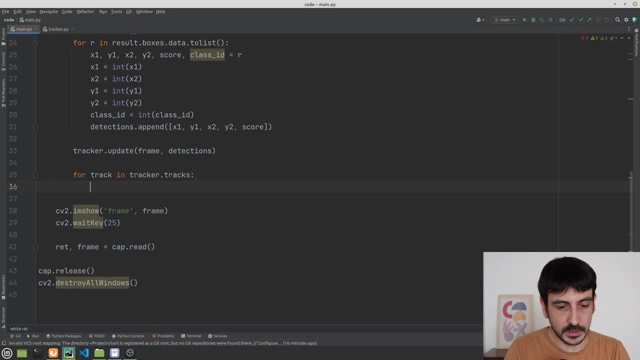 and this is what we are going to do. i'm going to access the track um bounding box- right, this will be the bounding box- and then i'm going to access the track id, which is the most important information from the object tracking algorithm, which is going to be the id, the tracking. 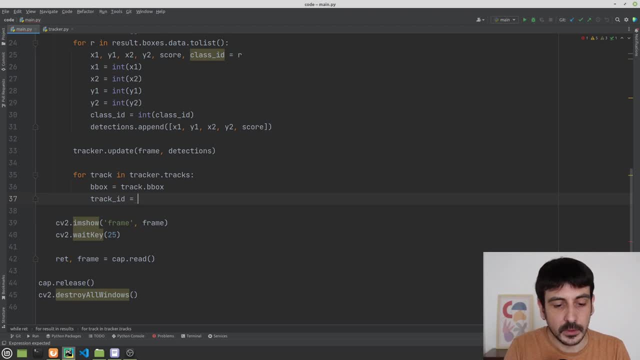 algorithm has assigned to this object, right, so track id will be track dot, track id. okay, and that's pretty much all remember. we are using an object tracking algorithm and every time we access one of these objects, each one of these tracks is an object. right, it's a, it's one of our. 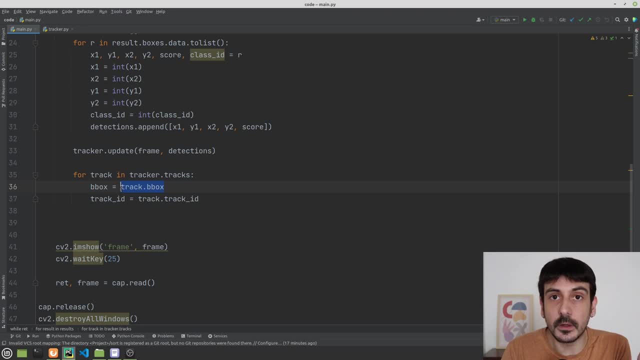 objects in the video and we are accessing the bounding box of that object in this specific frame and we are accessing the track id, the id the object tracking algorithm deepsort has assigned to this object right. the id will be exactly the same across all the frames in this video right. 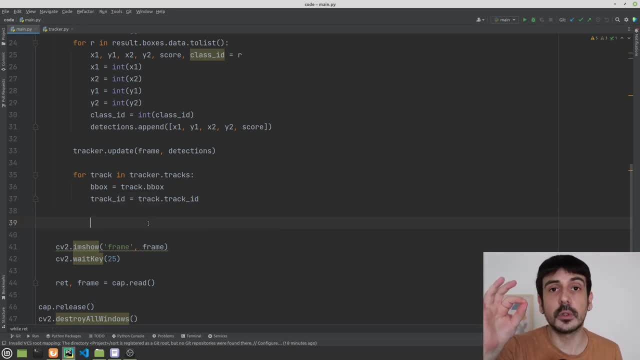 so each object, or actually each person, because we are already show you the video. this video contains people, and all the objects we are going to detect are people, are persons. well, we already know this. we are detecting birds also, for some reason, but it doesn't matter. most of the objects we are going to detect are people, and each one of these persons. 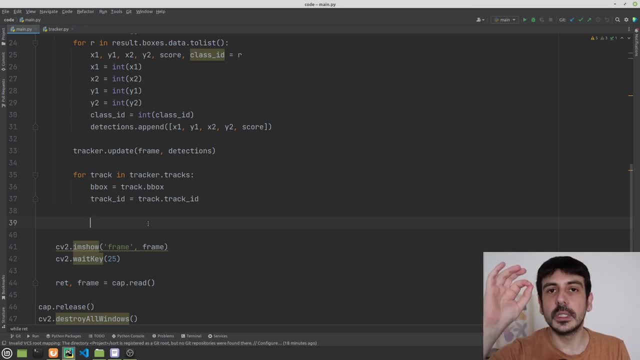 is going to have an id assigned. so the object tracking eye green deep sword is going to assign a given number, an id to each person is going to keep the same id across all the video, right? so absolutely all the frames in that video which contains that person will be with the same id. 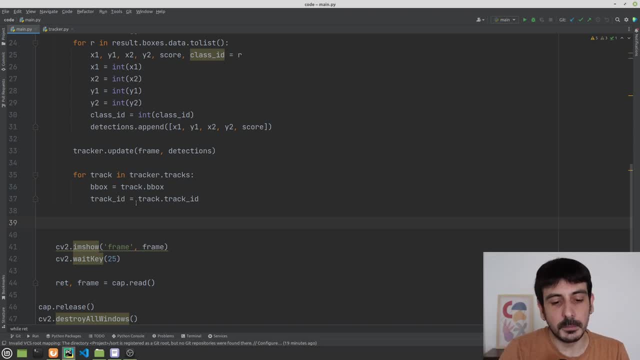 right, they will all be labeled with the same id. so the bounding box is like the specific bounding box of that person or that generic object we are detecting in that specific frame, and then track id is the id for that object or that specific person across all the frames in that video. so 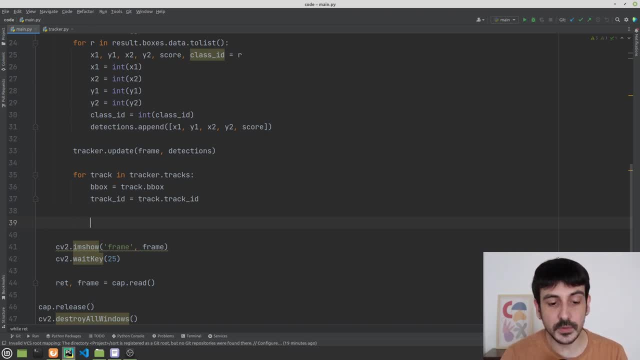 that's pretty much all for this tracking, and then what we need to do is to add a bit more. to do is just plotting a bounding box, a rectangle on top of the frame for each one of these objects, and so what I'm going to do is I'm going to define a new. 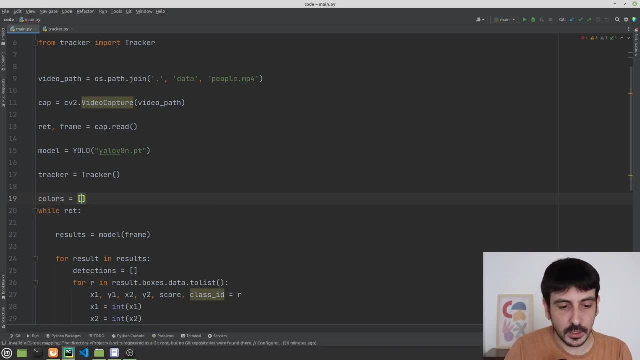 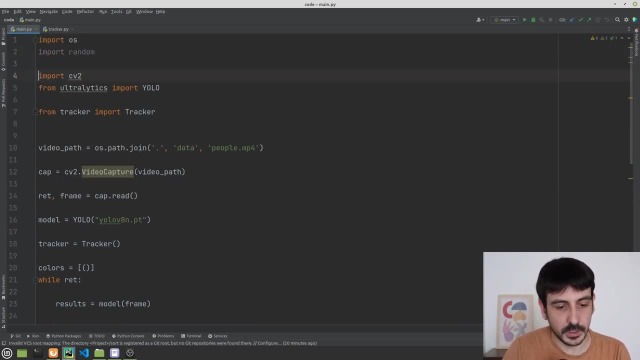 object, which is another variable, which is called colors, and colors will be something like this: I'm going to import random, port random, and then I'm going to call colors like randomrandint. this will be from 0 to 255 and I'm just going to repeat the same three times and this will be for jij in. 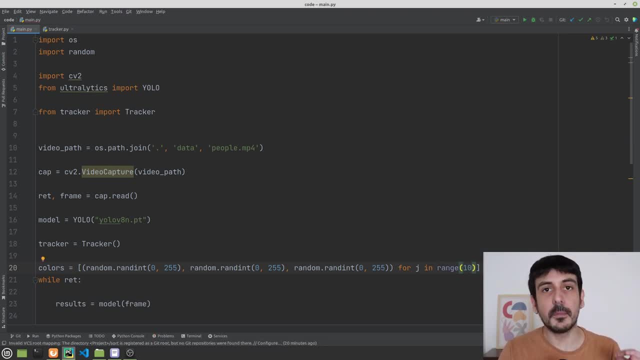 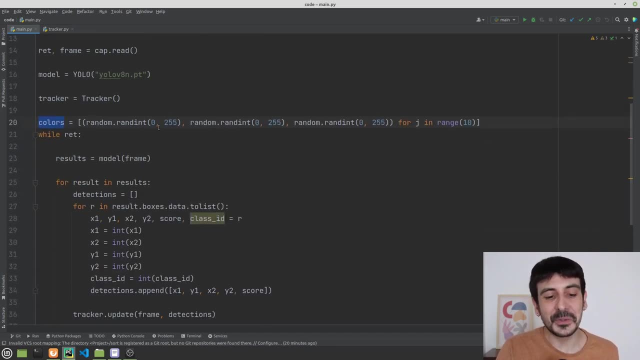 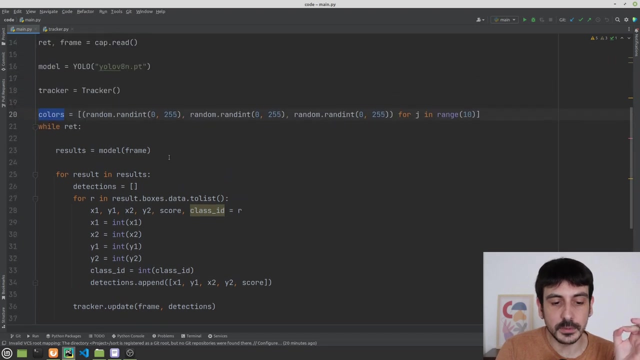 range I 10. so I'm creating a variable, i'm creating this list colors, which contains 10 completely random colors, and what I'm going to do is I'm going to plot each one of the first Persons in the video I'm going to choose. I'm going to plot each one of these persons with a different color, right? 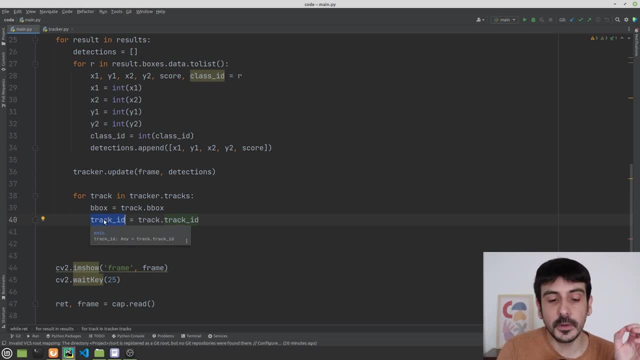 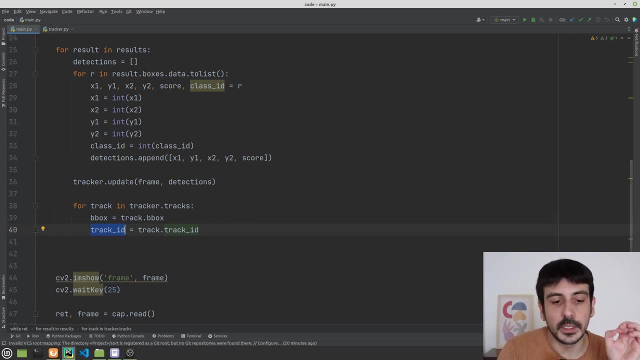 So, every time we get a new ID, every time we get a new identifier, We are going to plot this new ID, this new object We are detecting, with a new color, right? We are just going to select another color from this list, right? That's the idea of what we will be doing now. 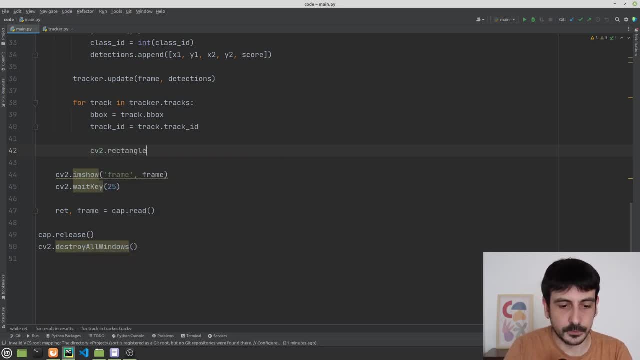 so I'm just going to call CP to rectangle and Now I will call, I am going to input the frame and then the top left corner, Which will be x1, y1.. I haven't defined what is x1- y1, but it's basically x1. 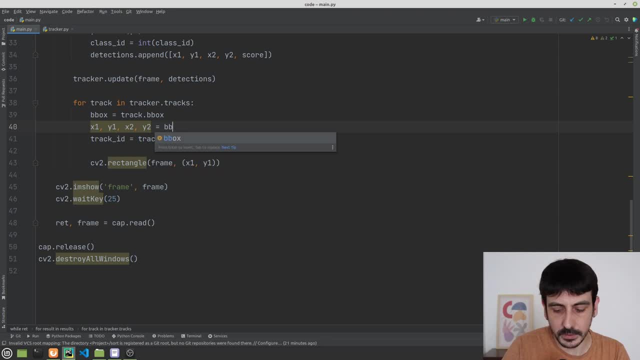 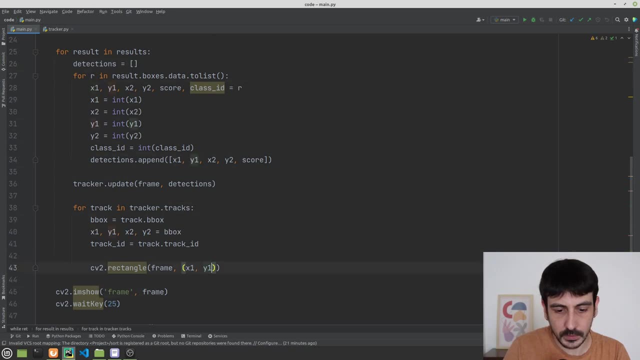 y1, x2, y2- this is bounding box, Right, And then I am going to Do something like this: This will be x2, y2, Which is the bottom right, then the color, which will be colors, then the track ID, But divided, or actually mode Mode. 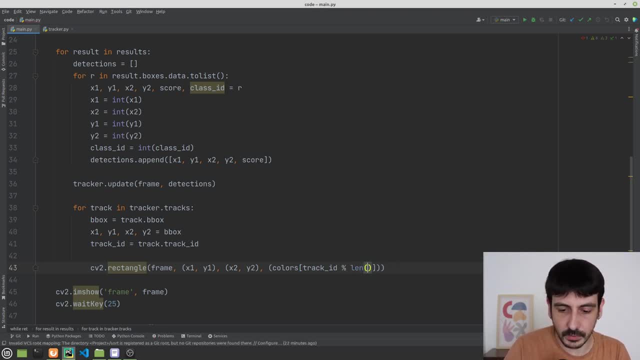 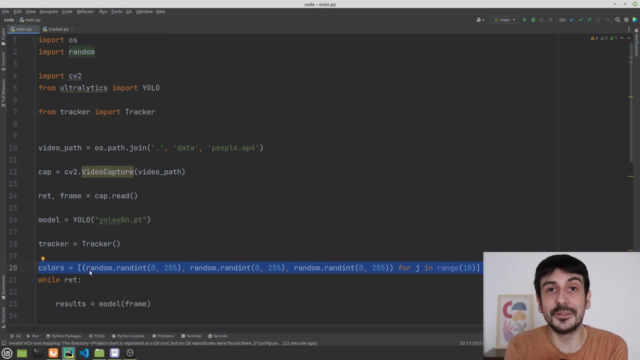 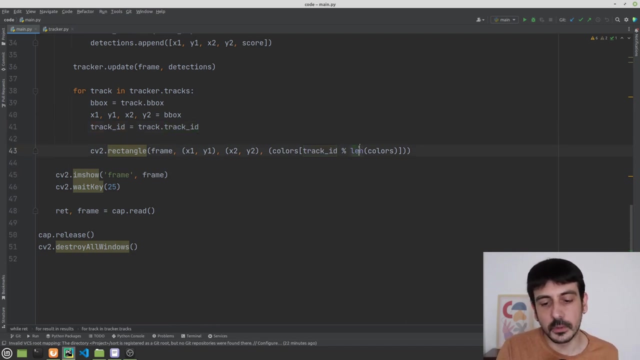 The length of colors. right, Because, remember, these are right. this list Has only 10 elements and we will be detecting many, many, many, many, many many objects. so this track ID Will have a value which is super, super huge, and if we don't do something, it is we are just going to. 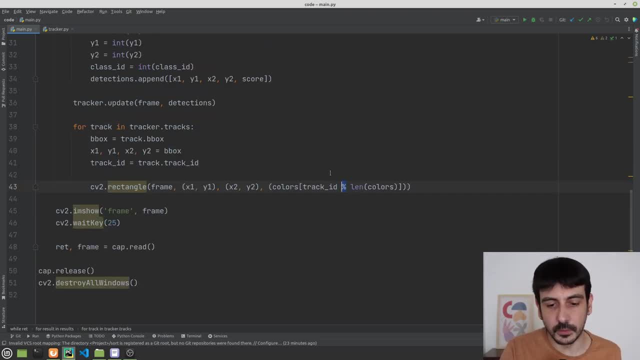 Get an error right, So we definitely need to add this mode to make this work. Okay, Now that we have specified the color, And the only thing we need to do is to specify the width for this rectangle, and that should be all, and let's see if we are. 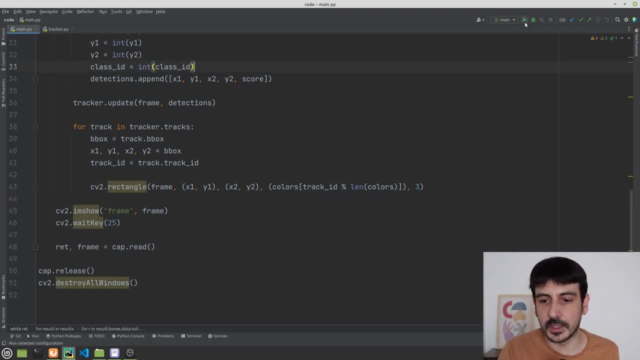 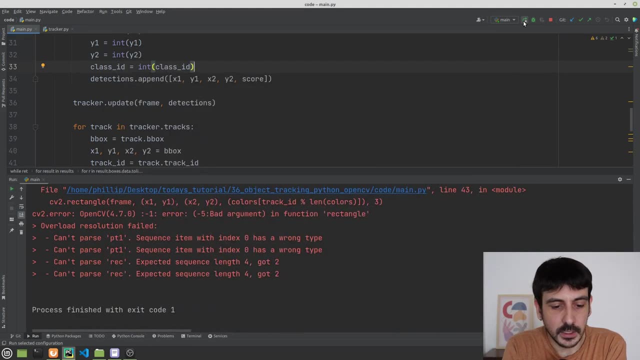 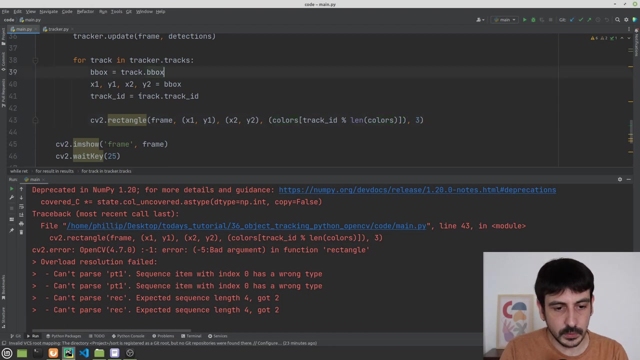 Doing everything correctly. Let's see if we can. just let's see what happens if I press play now. We should be looking at our frames just like before, But we should be getting a bounding box on top of our frames and we're not getting it, So we have done something wrong. Let's see What is it. We may need to cast this as an integer. 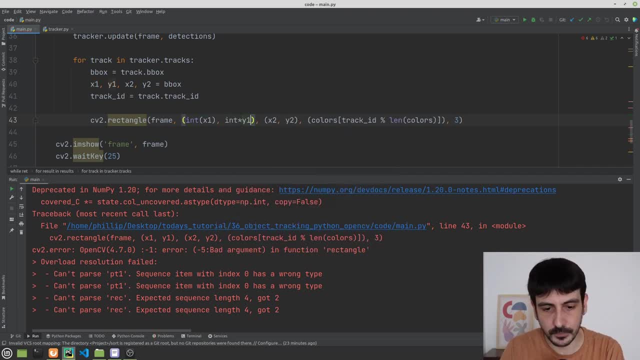 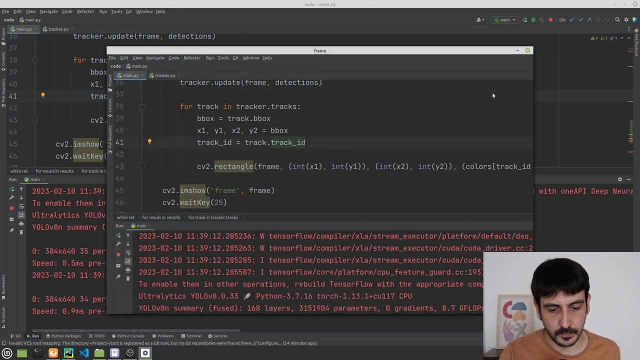 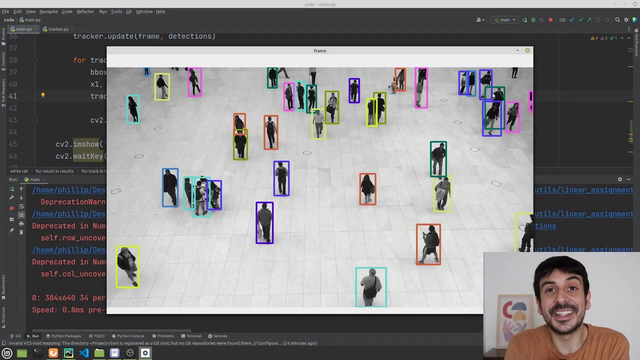 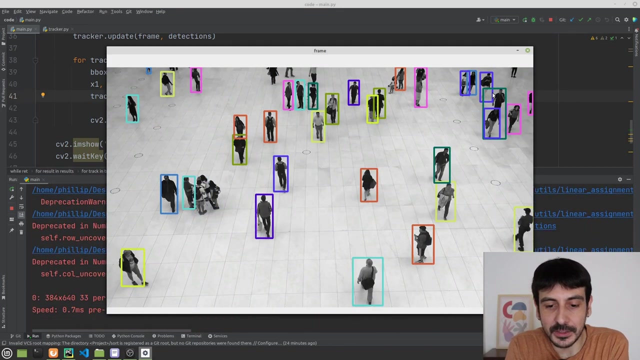 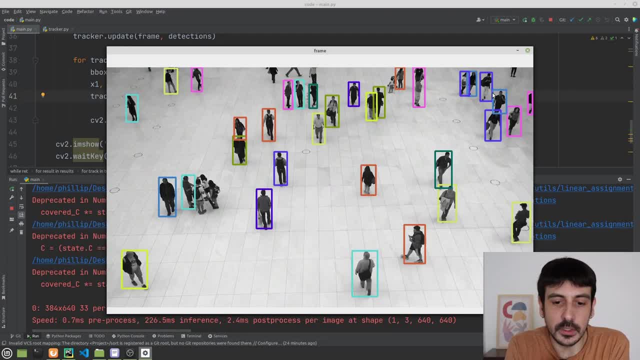 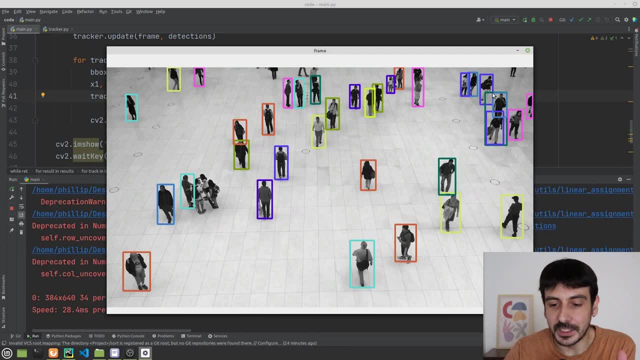 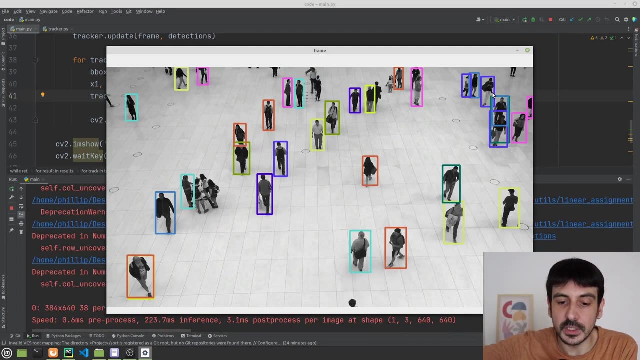 obviously We are executing the sort and we are also executing yellow V8 and we are running everything on a CPU. So we are not getting a real time detection and And we are plotting many, many different objects. So DeepSort is computing different features and doing different things for each one of the objects you can see in this image. 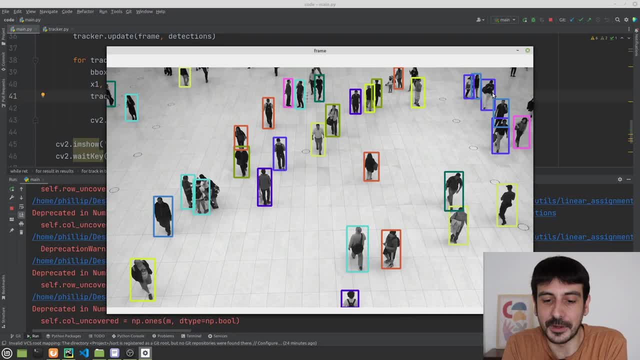 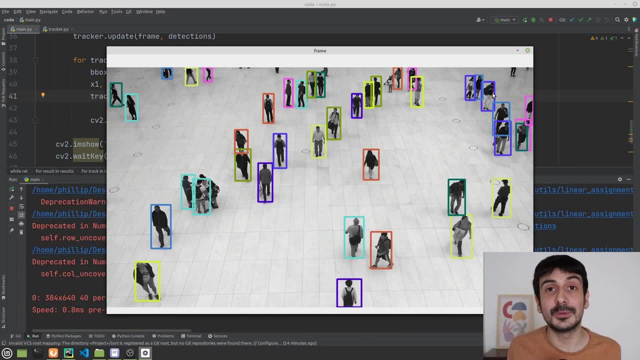 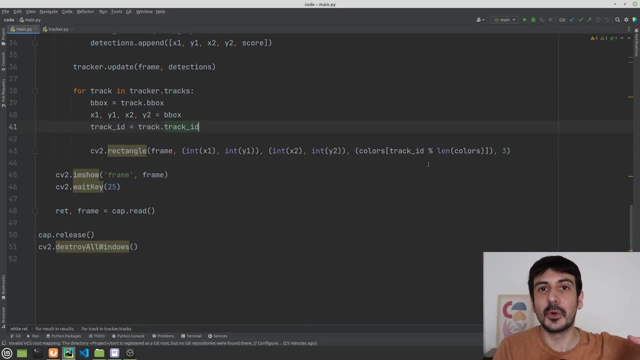 So, yeah, we are doing many, many, many stuff. We don't have a real-time execution, But nevertheless, you can see that everything seems to be working just fine. Everything seems to be working super, super, super properly, So the only thing we need to do now is to save this video back to our computer. 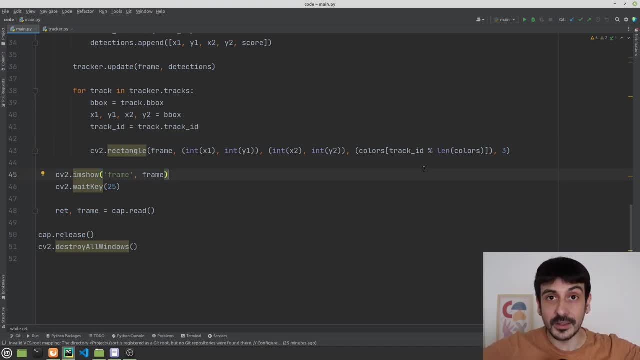 We have already solved this problem. Everything is ready. Everything is absolutely solved. We have implemented the object detection using YOLOv8. And we have done the object tracking using DeepSort. So everything is ready. The only thing we need to do now is to save the video back to our local computer. 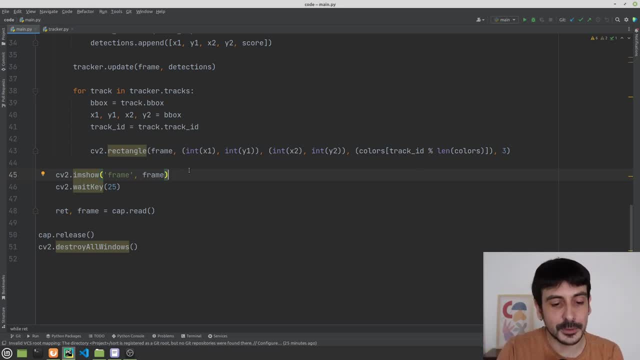 So we have the video with all the different frames and with all the different detections and so on, And we can analyze this video in a much better way if we have the file in our computer. But everything is ready. We should be super, super super happy with ourselves because we have solved the problem already. 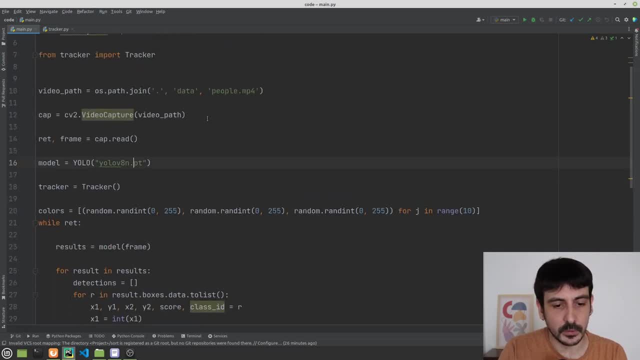 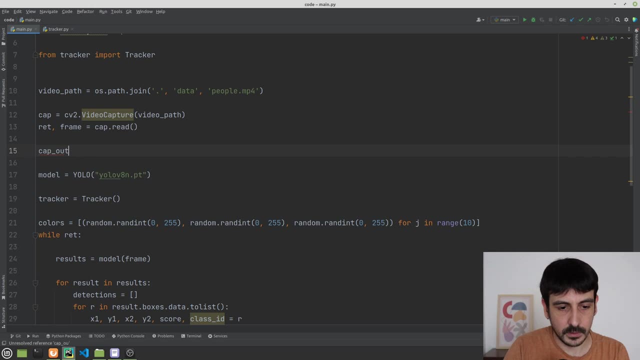 And what I'm going to do is I'm going to create a new object, I'm going to create it here, I'm going to create it here, which is a cap out, And this will be CB2 Video Writer, And I need to specify the location of where I'm going to save this video, which maybe I can say something like: 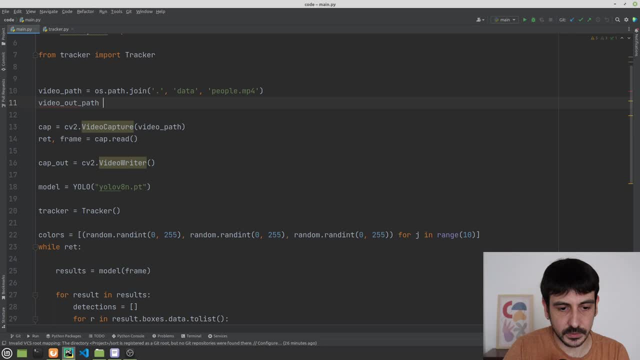 Video Out Paths. I'm just going to save it in my local, in my current directory, And I'm going to save it with the name Outmp4.. It's exactly the same. You can choose another name. You can choose another location. 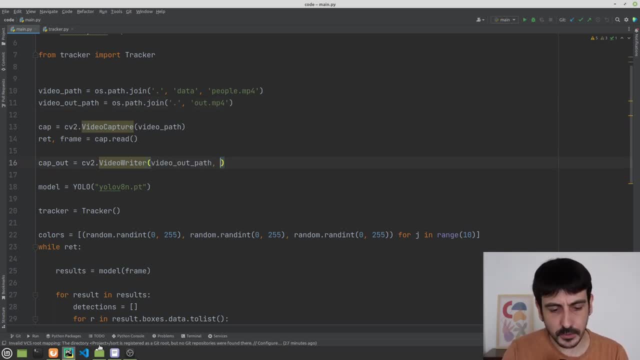 But it's exactly the same, And now we need to input a couple of values. And now it will be much better. if I can just look at this file, These are the choices. These are the two values we need to input. You can see, this one is related to the codec we are going to use in order to write this file. 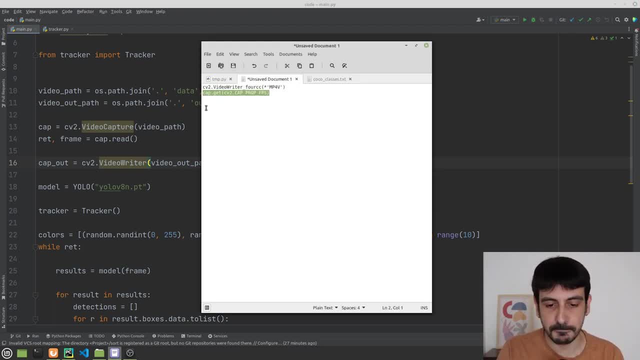 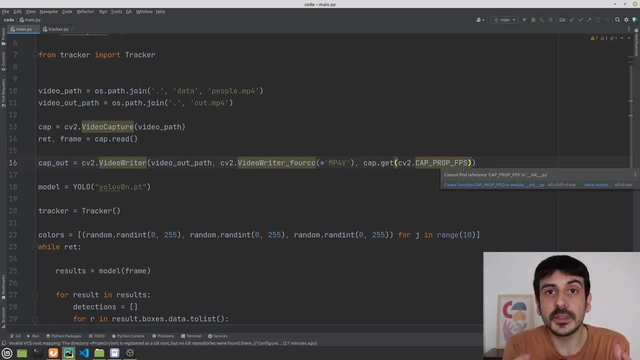 We are going to write an mp4 file, So we definitely need that value. And then we need to specify the frames per second in this video, right, And we want this output video. We want this video we are going to write into our computer. 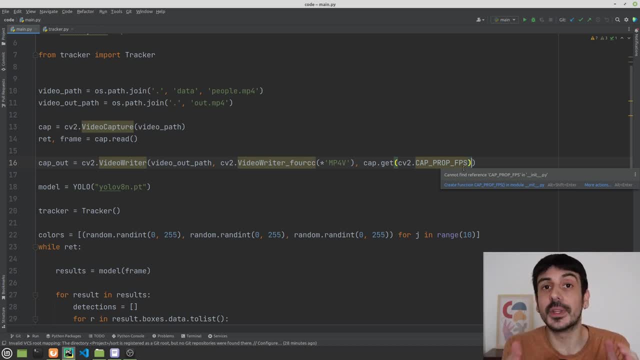 We want to make it the same frames per second as the original video. That's what we want. So we are going to call cap, which is this object, the video we are reading. right, This is the OpenCV object for the video we are reading. 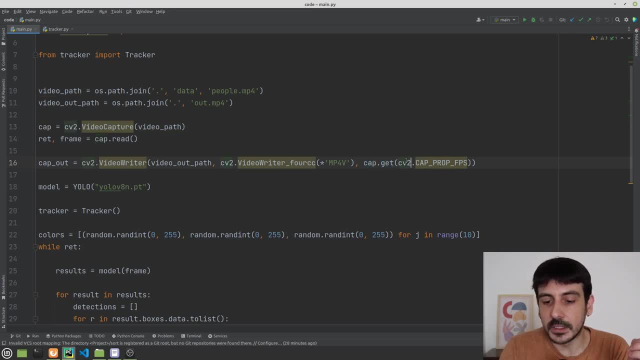 And we are going to say: capget this constant. So we are getting the frames per second of the original video. That's exactly what we are doing here: We are getting the frames per second of the original video. So we are going to make the output video, the video we are going to produce. 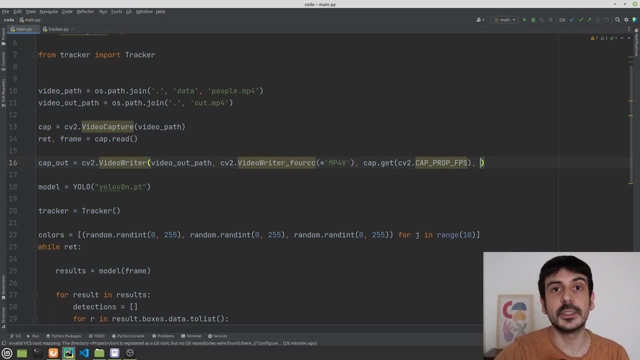 we are going to make it the exact same frames per second And we are going to say frame rate as the original video, Which is a very good thing because we want to have, like a real experience. right, We want to look at this new video and we want to make it as similar as possible as the original video. 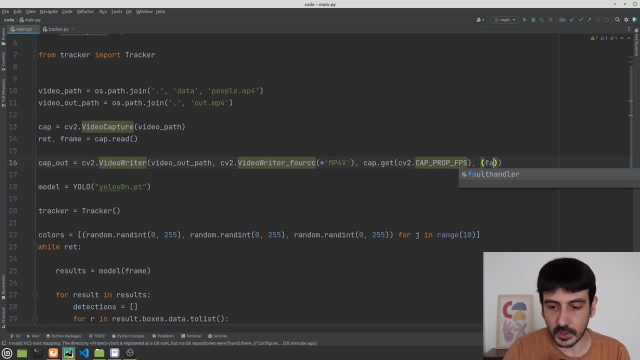 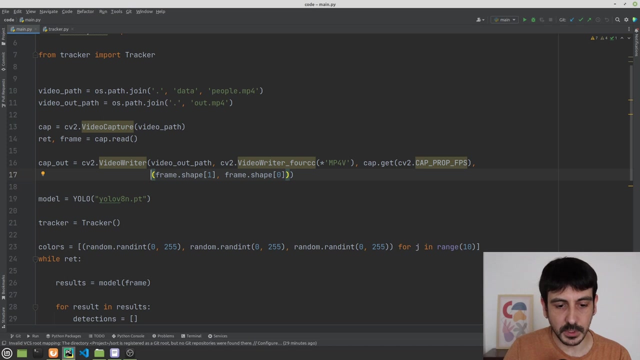 And then we need to specify the size, And I am going to say this will be frameshape 1 and then frameshape 0. And I am going to press enter, Okay. So that's pretty much all, if I am not mistaken. 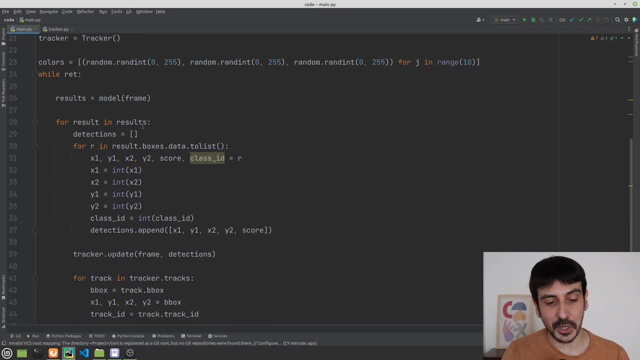 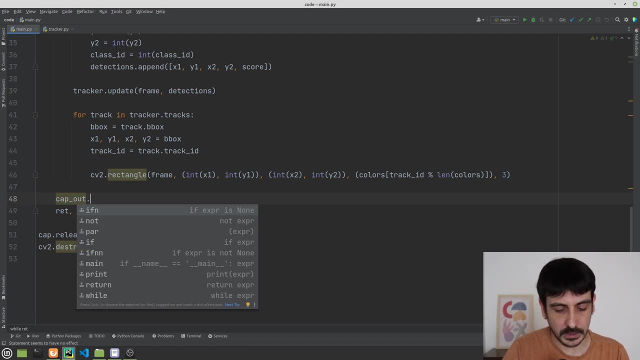 So I am just going to take this cap out, I am going to take this object and I am going to write the frame here. Just before I read a new frame, I am going to write the previous frame And the previous frame. you can see that it's the one I have just draw all the rectangles on top. 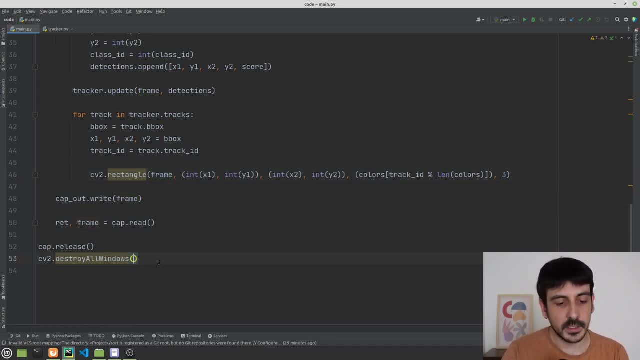 So this is exactly the frame we need to write, And now I am going to release the memory, The memory from cap out 2.. And that's pretty much all So, if I am not mistaken, this is pretty much all I am going to press play. 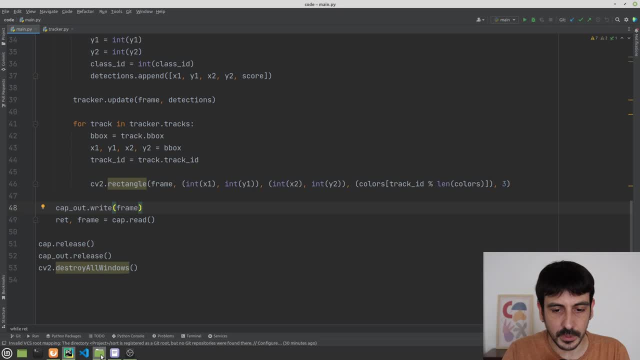 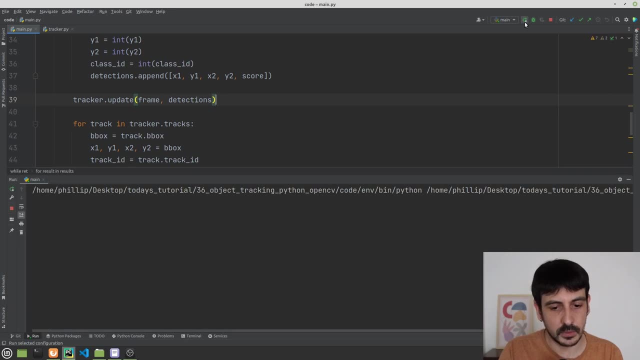 I am not visualizing the frames anymore. If I go to a local, if I root directory, I don't see any file, anything. So if I press play, everything should work just fine. We should have a huge output with a lot of warnings, a lot of everything. 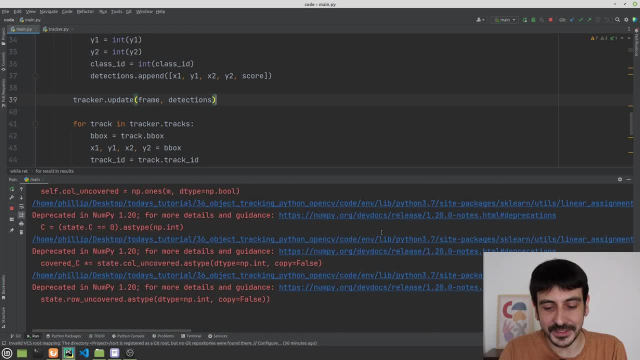 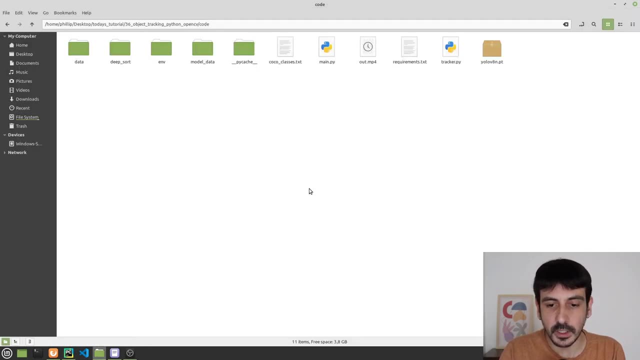 Just ignore all the warnings. They don't really mind in this case. So we are getting a lot of outputs, but nothing is going on. We are not getting any error, And if I go back here, you can see that a new object called outmp4 has been created. 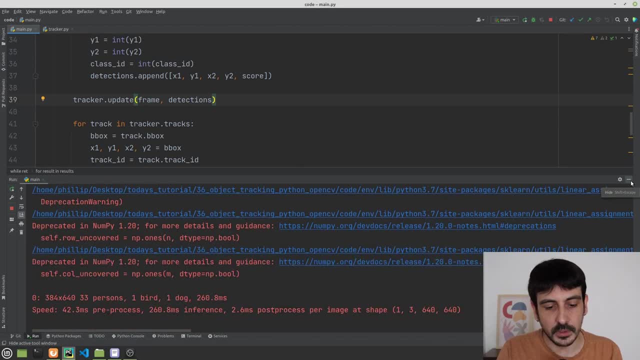 And it's just writing all the frames in my code. So now the only thing we need to do is waiting until this code executes absolutely all the frames, And it just writes absolutely all the frames. So I am just going to pause the video here. 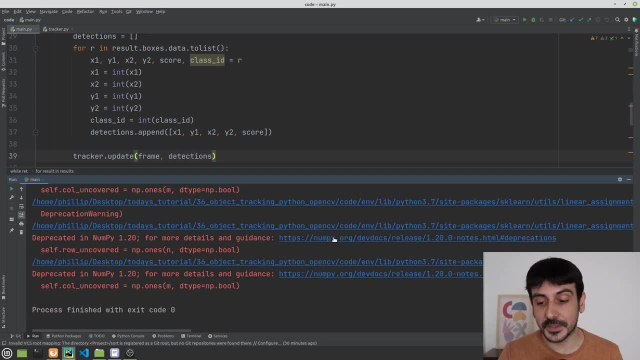 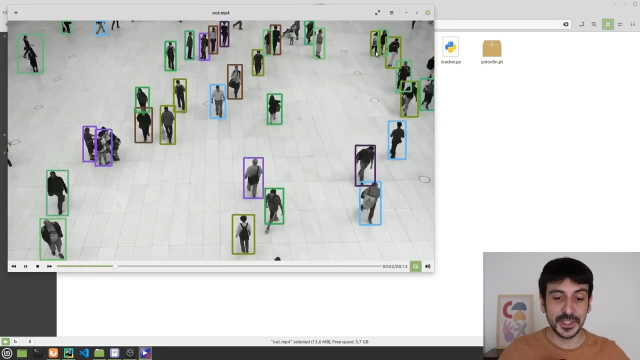 And I am going to fast forward when this is completed. Ok, so the execution is now completed And let's see our video. Let's see how our video looks like. This is the video we have generated, And you can see that we have different colors for different IDs. 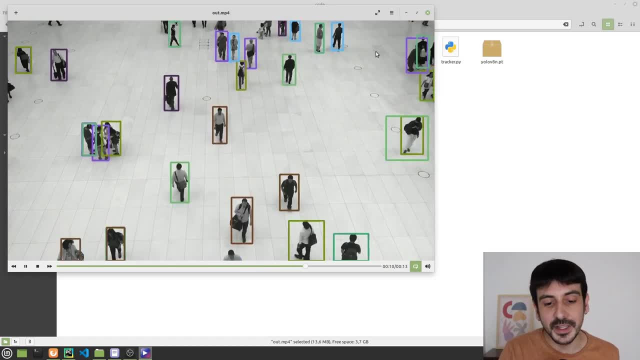 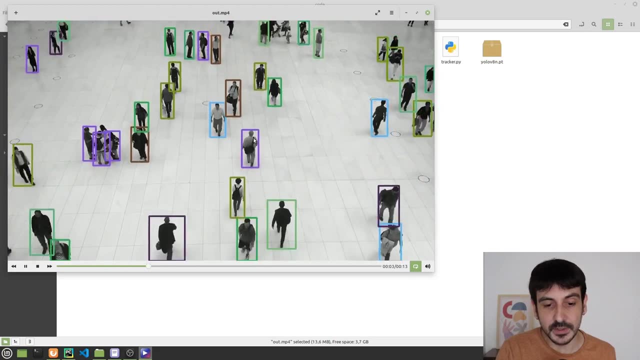 For different objects or for different people. we have detected And you can see that it is working pretty, pretty well. If we look at, for example, this person, You can see that it is a very stable detection. We are detecting absolutely the same person in absolutely all the frames. 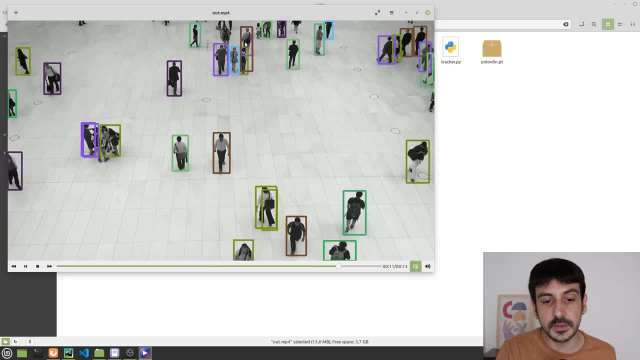 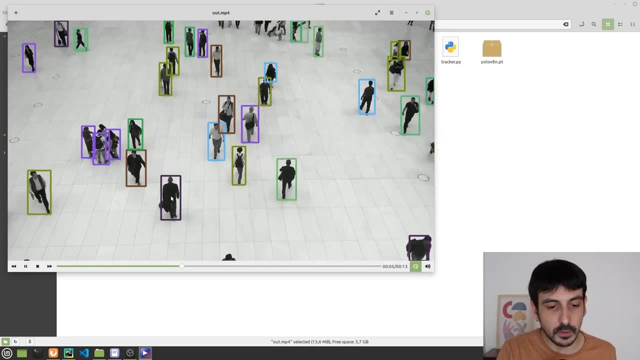 The color is always the same. If the color is always the same means it hasn't detected this person as another person, But it is always the same person And the same happens with absolutely all the people I am seeing over here. Maybe there are a few misdetections. 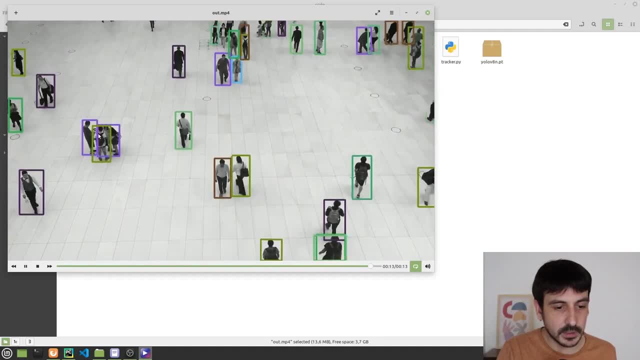 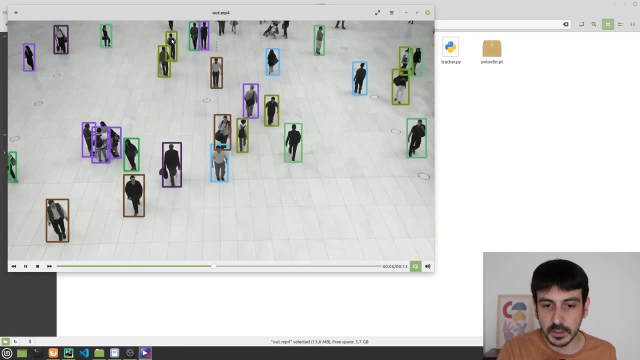 For example. here you see, it goes a little crazy. The detection is not 100% proper And there may be some more misdetections, maybe over here And maybe in those cases where we are not getting a good detection- But nevertheless I would say this is a very, very, very good result. 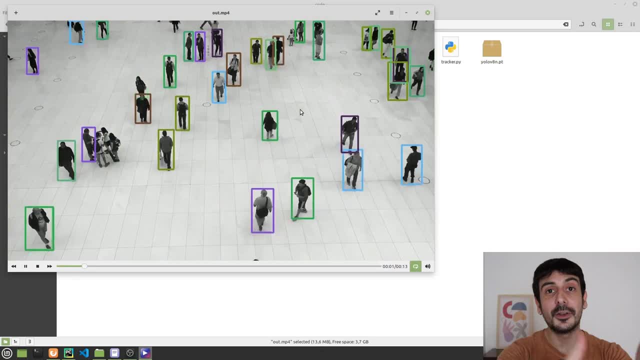 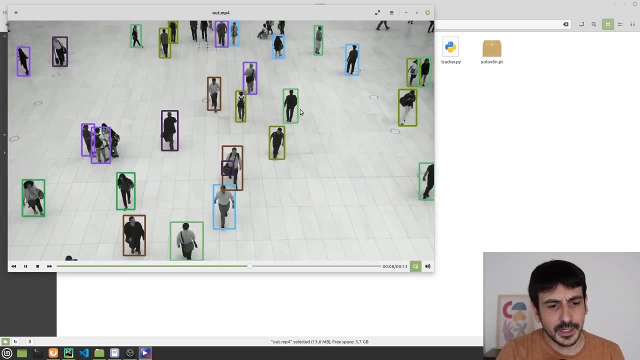 So this is going to be all for this video. This is exactly how you can implement an object tracking algorithm using DeepSort, Using an object detector as YOLOv8.. Right, And now that I realize, I see that we are only seeing people. 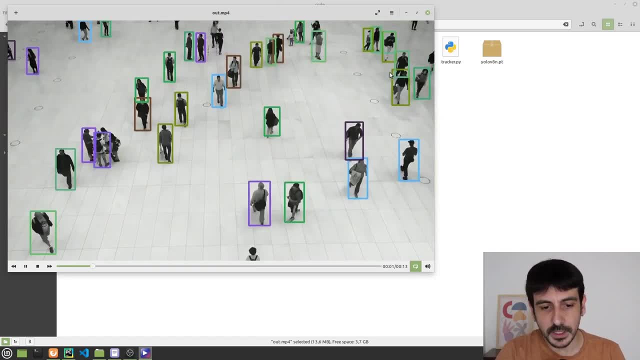 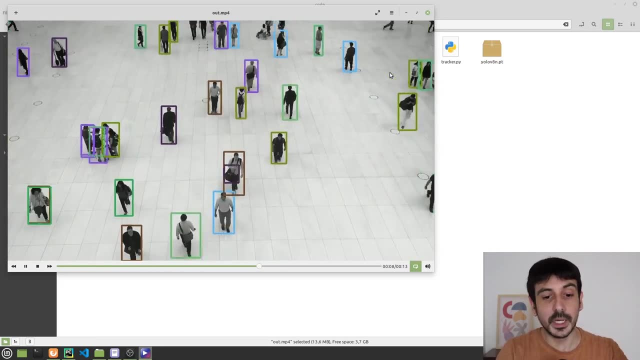 We are only detecting people And I don't see any bird through the entire video. Right, Maybe I am missing the bird. If you notice the bird, please let me know in the comments below. But I don't really see it. But you notice, in the detections we were detecting a few birds.